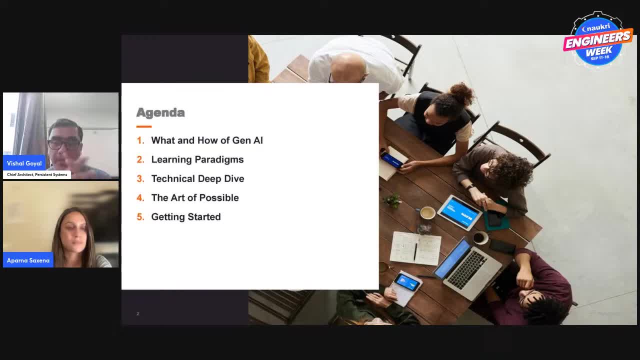 these important areas. So what Gen AI is? a lot of you may know what Gen AI is, but I'll go a little from beginners on how this has originated and why this hype now versus last year. Then what are the different ways of how people are looking at Gen AI? We'll do a little technical deep dive for 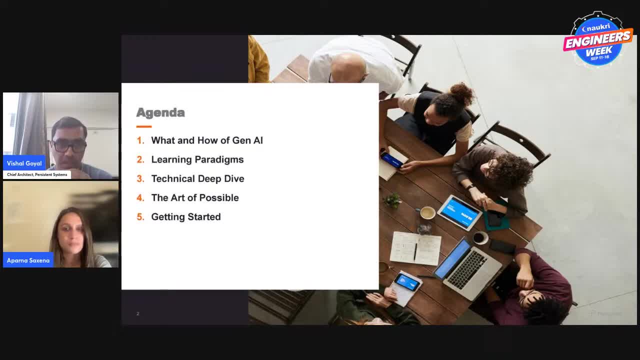 audience on the call, who are already knowing what Gen AI is, to know what topics, what areas of Gen AI should people be aware of, what skills to be built. And then we'll go to the core of art of possible. I want to show you areas of Gen AI and areas of software engineering which can 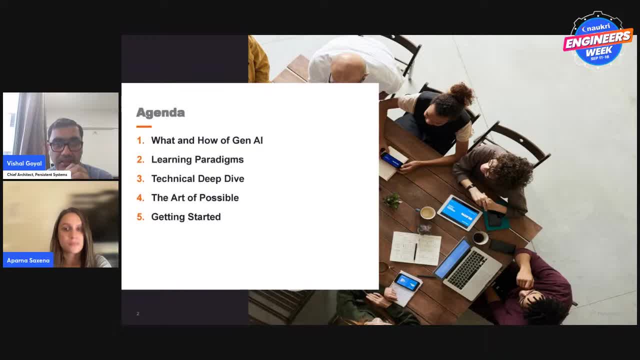 be really done with Gen AI with relatively ease, And then at the closing I'll have some getting started notes for people to know how to start which training courses to do and so on, And then we'll open up our questions and any any. 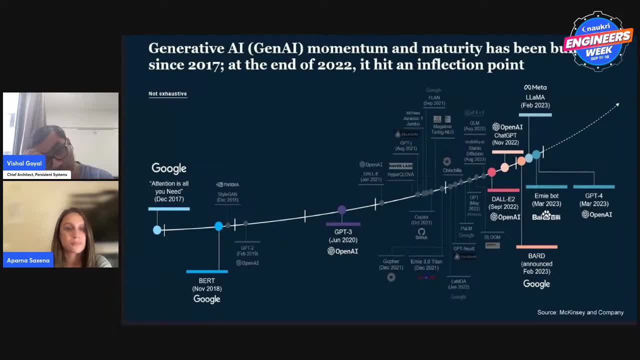 any questions that people have. Okay, Now, if you look at Gen AI, right, it is not something which is new. AI has been there in existence for starting from 2018, which is where Google released their birth model open source date. Then 2020 is when GPT came in play and open AI really started making a good impact in this whole space. But still, if you look at 2020, I know COVID happened, but nothing really happened much with even with GPT. 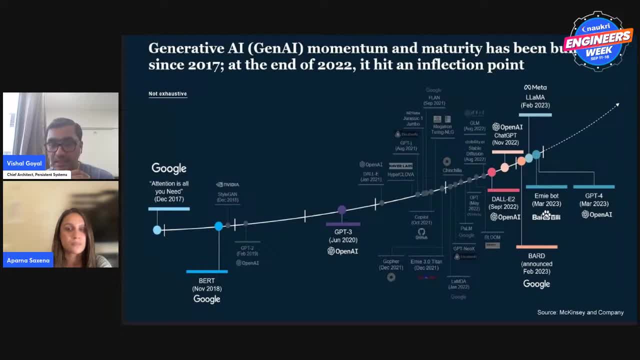 People were doing bits and pieces of work but nothing, nothing extraordinary, was coming out of it. Chat GPT happened somewhere last year and that's where things have exploded completely Right, And that's where we are calling it an infection point. After chat GPT came in and people realize, oh, I can talk to data as a normal human being. I can get into a conversation And the person who I'm talking to remembers, like I'm talking to Aparna right now. Aparna will remember the conversation and she'll have a context to it. That's what I'm talking about. 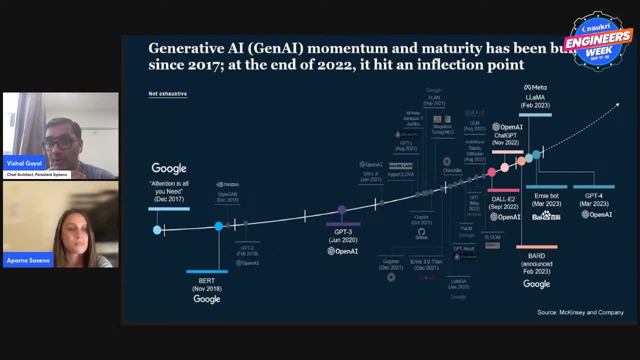 Right And all of a sudden everyone was kind of hooked on to Gen AI and understanding what it can do. And then if you see, in last six, seven months things have just completely exploded. Right, What chat GPT came in. this was GPT 3.5. It was only text based communication, but then open AI launched GPT 4.0, where you can do much more. It is multimodal, You can do images, you can do videos, you can do music. 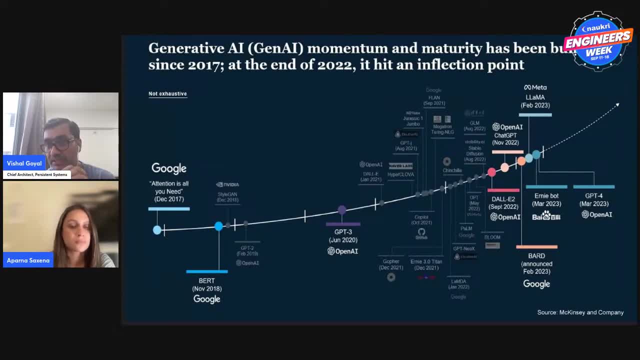 A lot of applications have got released after, And that's where everyone on this planet today is looking at Gen AI, on how Gen AI can solve, not just in software engineering different areas, but how Gen AI can be used across different industries, And we'll look at some use cases as we move along. But the advertising industry is using it, The healthcare industry is using it. You call it, banking industry is using it. 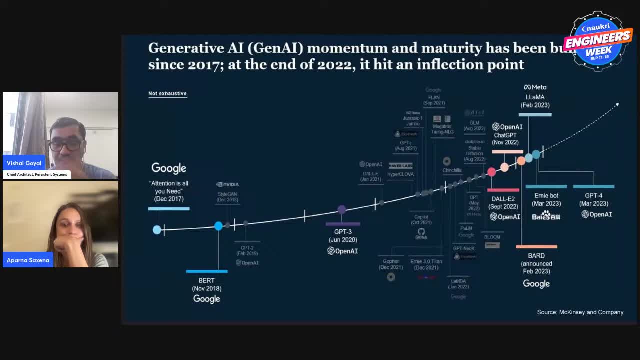 The content generation has become so, so easy with chat, GPT, on how, In general, with Gen AI, whether you use chat GPT, whether you use Google board or anything else right, And GPT 4.0 has completely changed the dynamics. 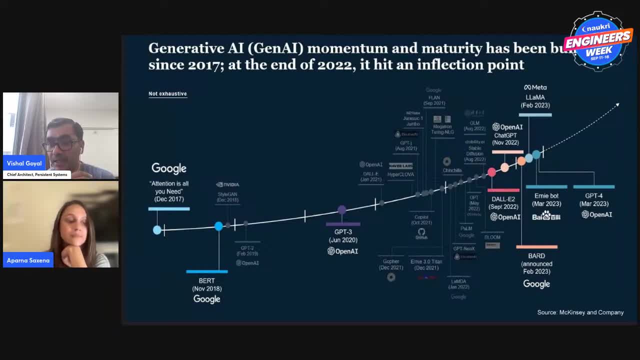 If you hear the CEO of open AI- he was here in India, there was a session done- You would realize that they don't want to open out GPT 4.0 because they fear that if people know what GPT 4.0 can do, people will start misusing it as well. 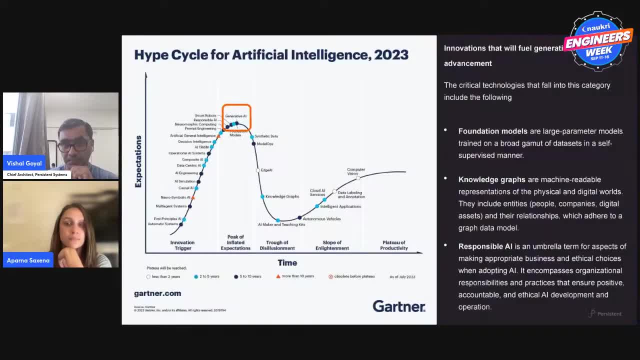 And we'll see some of the pitfalls of Gen AI as well. So that was the origination of Gen AI, Right? So that was the origination of Gen AI, Right, So that was the origination of Gen AI. But if you look at Gartner and the hype cycle of AI for 2023, this is just released a few weeks ago. 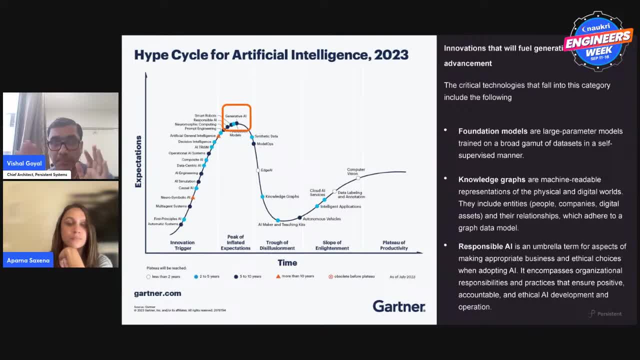 You see, Gen AI has already crossed the innovation trigger, So people who are not knowing what Gen AI is are probably already way behind the curve in terms of where they should be. Gen AI is already at a peak of inflated expectations now, And within the next five to 10 years, we expect this to really be a game changer in terms of how people are using Gen AI. 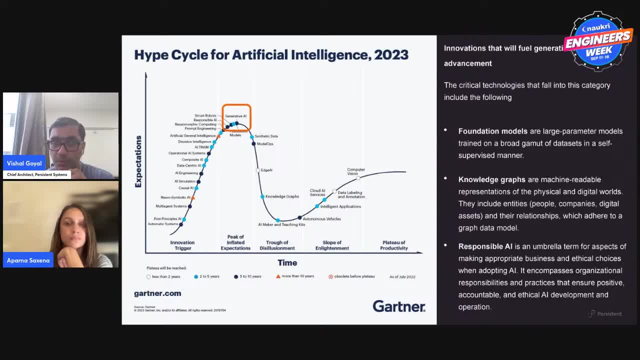 And a couple of points from the Gartner- and people can go to this Gartner hype cycle and read more about it. But foundation models, which we'll talk a little bit more, knowledge graphs and responsible AI have become extremely important areas of Gen AI. 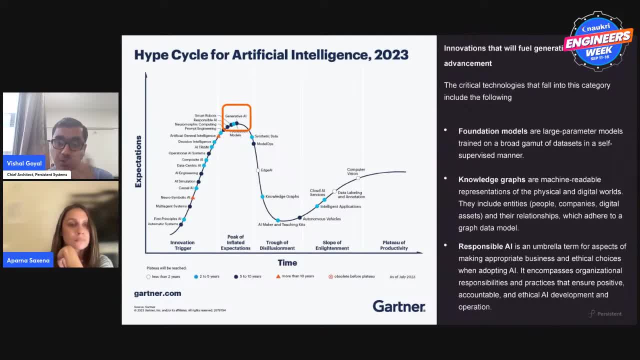 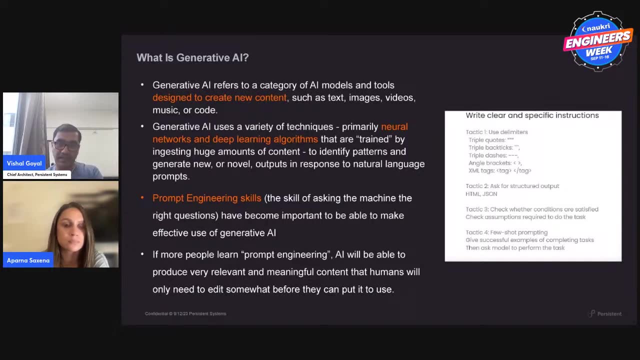 Responsible AI is again very, very important that, while you use Gen AI, your user responsibility, which was always the case, even with the core AI. for many, many years Now, what is Gen AI? People have been saying- and I don't know if people follow me on LinkedIn, but I wrote an article a few weeks ago to say we had Gen Z and we had Gen X. 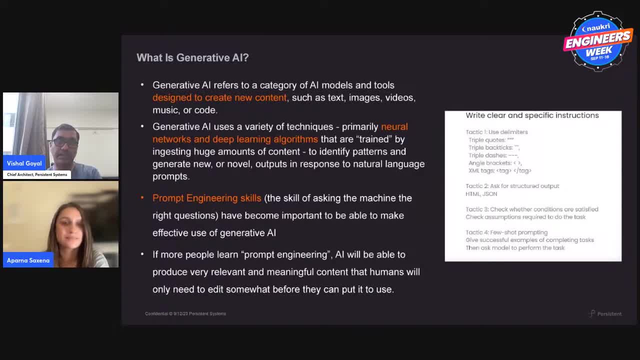 Now we have Gen AI. That's how the new generation of people we are creating today. So it's basically a category of AI models. AI always existed, but this is essentially saying it is designed to create new content. You had AI which was supervised learning, unsupervised learning, and then you had reinforcement learning. 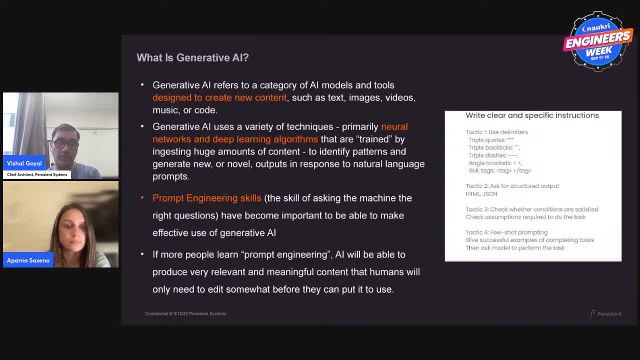 There was a way on how you train the model and then it will work, and we'll look at it in a little bit more detail. But this one is basically: you don't need to train it. It will create new content for you, whether it is text, images and videos, and this essentially uses the same neural networks and deep learning algorithms behind the scenes. 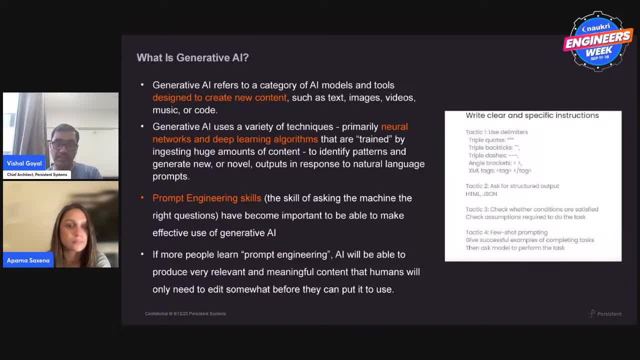 What has come out very clearly is a new skill which everyone needs to know. who needs to work on Gen AI, which is prompt engineering, Prompt engineering, nothing. but how do you talk to me or talk to someone else? So you talk in a natural language. you will ask a question, you will react to my response, you will again do a follow-up question and you will react to it. 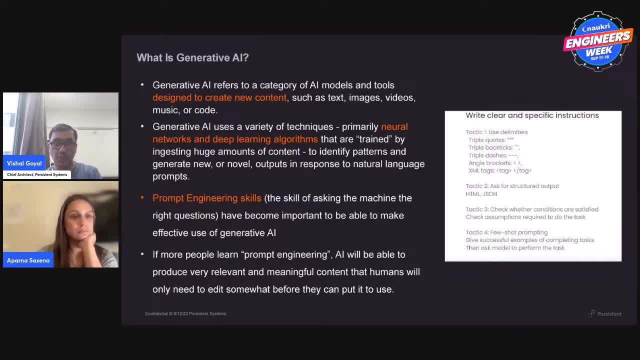 That's what essentially prompt engineering is. in very simple language, You need to know what to ask ChatGPT for it to be able to give you a response, And if you don't ask the right question, it will not give you the right response. 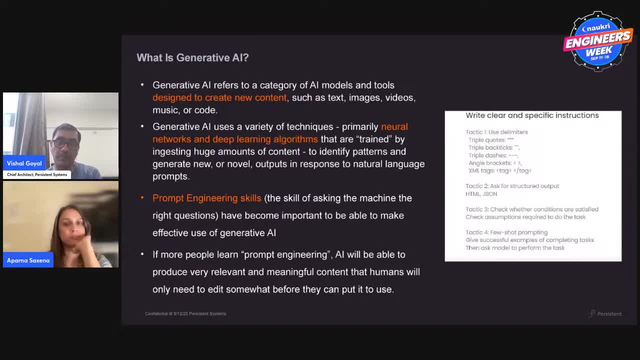 And there are different areas of prompt engineering. People would have heard zero-shot prompt engineering, few-shot prompt engineering. That's the different technique. So if you were to say: where do you want to go, Where do you want to go, Where to start from? 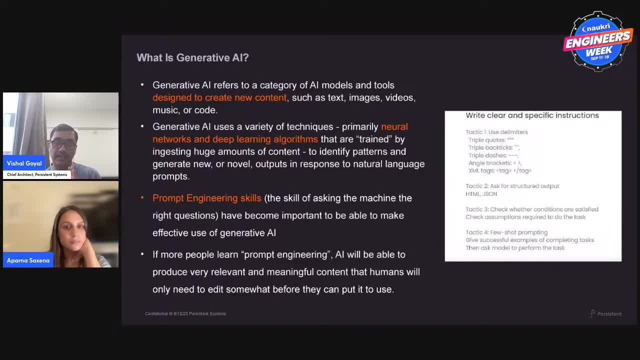 And what is the most important thing, which people should do before they look at Gen AI, They should do a course on prompt engineering And at the end of the session I'll have some pointers on what people should do with prompt engineering. But if you look at resumes today, people are saying they have an expertise on prompt engineering on a scale of one to five. 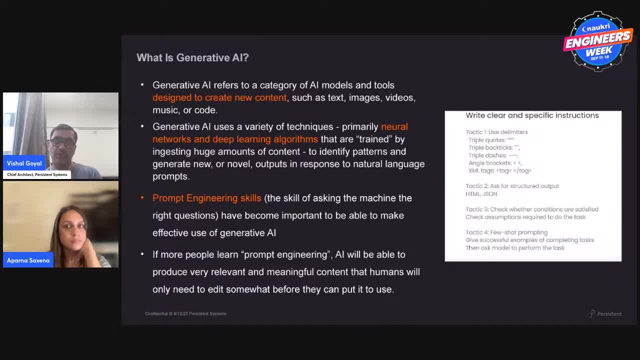 Like they would say, I know Java and I'll rate myself three on a scale of one to five, five being the best People are saying. I also have prompt engineering skills now And I would rate myself two or three or even five. 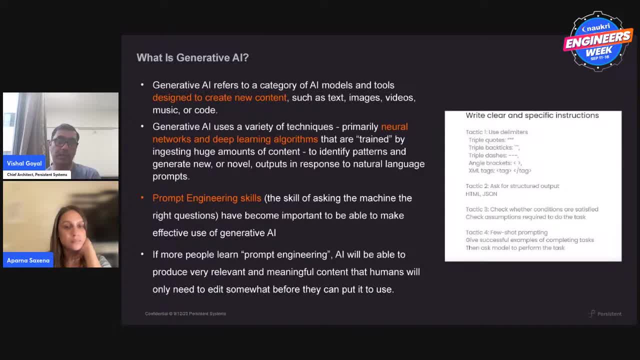 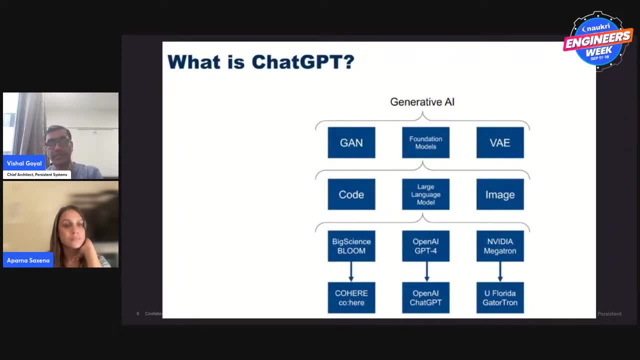 And I know how to write prompts and how to change those prompts and how to basically do prompt engineering. So what is TagGPD? So you had GAN, which was Generative Adversarial Network. You had a lot of other stuff. 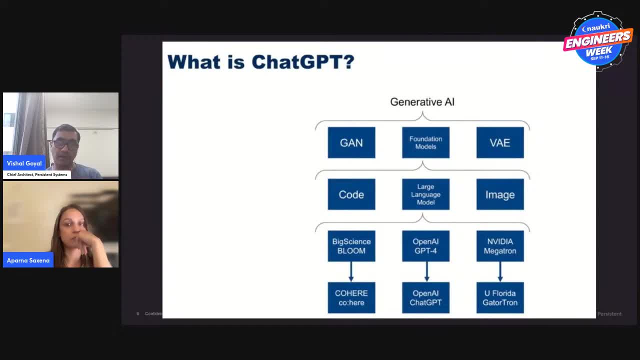 And then you had something called foundation models, And foundation models could do a lot of things. So you had DLA-E2, wherein you could give a text and it will generate an image, which is one kind of foundation model. And then you had something called large language models, which is an example of what OpenAI and TagGPD and GPT 3.5 and 4 does. 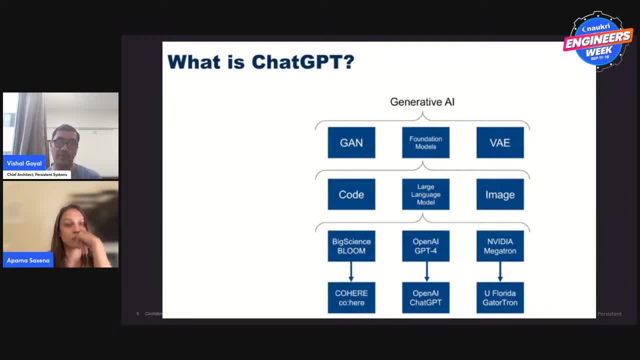 And that's where large language models came in. And then you have a variation of that with OpenAI. And then TagGPD is nothing but one of the applications of OpenAI. It's an application which has been built. It uses GPT 3.5 and now GPT 4,, the commercial version. 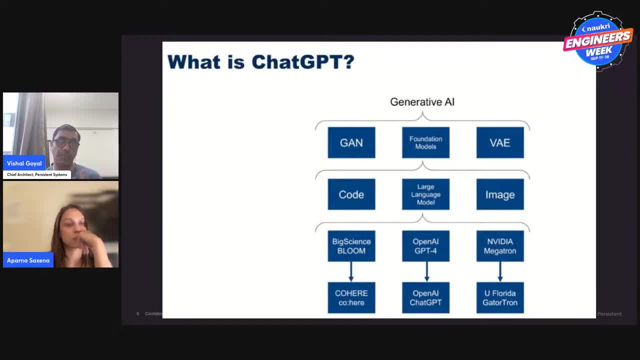 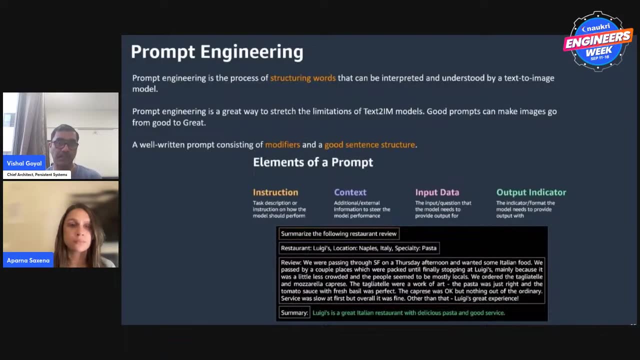 And that's what TagGPD is right. So it's important for people to know that, That how things have moved from the traditional AI into the GenAI, And how foundation models, large language models, LLMs fall into, And then how TagGPD links to all of these. 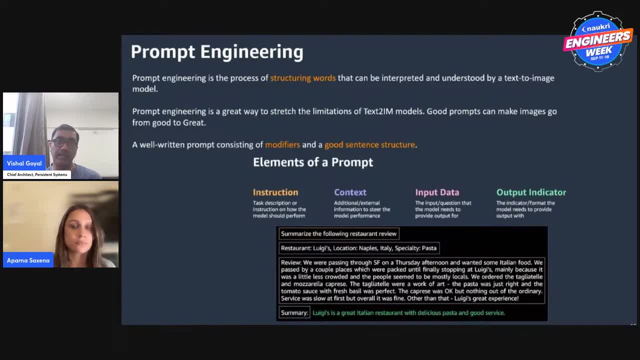 I spoke about prompt engineering, Very important skill. People need to know how to write a prompt, So it's basically an instruction which you give to an interface. So if you are using TagGPD, it's a UI interface, But if you are using something like LLM models in AWS or Azure or OpenAI- 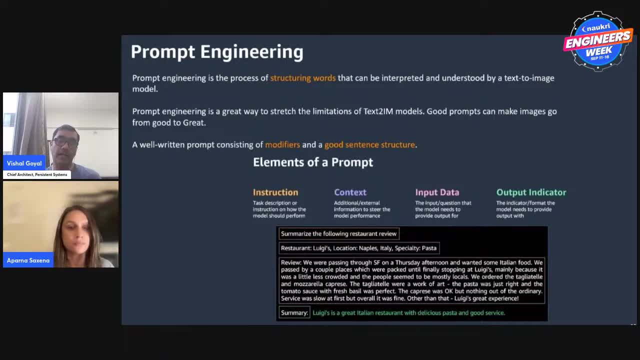 it's not a UI interface, but it's an API call And to an API you give an instruction that I want you to do this, Whether you want to convert a program from one programming language to another or anything else- And you have to give a context so that it understands what you want it to do. 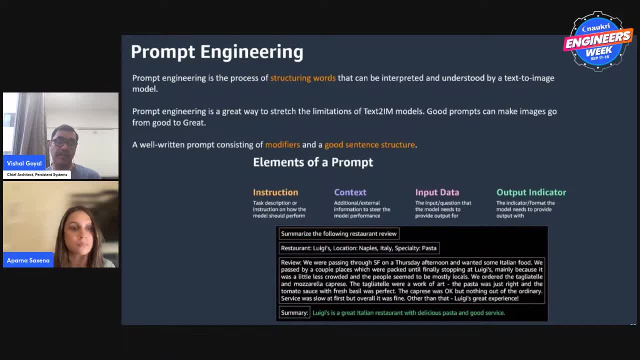 So you may say: I am a senior architect and I'm trying to build an application. I want you to help me understand if it's an e-commerce application where I want people to be able to do stuff what it should do. That's the context. 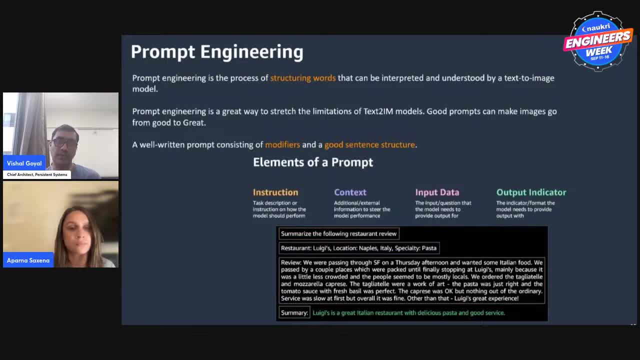 And now, if you see TagGPD, it also has a settings where you can say, you can give your profile to say: this is who I am and this is what I expect. So every time TagGPD will generate a response, it will keep that context in place. 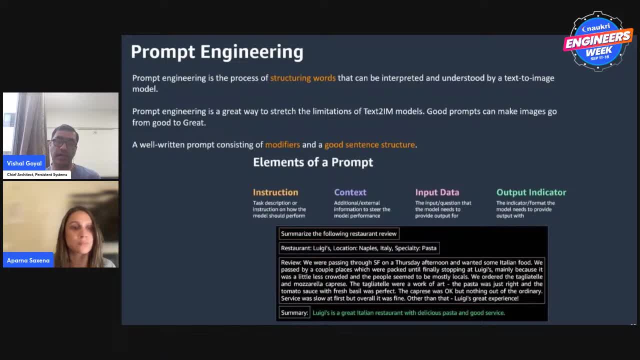 They give a question. That question goes through a large language model. It does the prompt. engineering creates the prompt, gets you to the output, And that output is not just like a one time response. You can then do a conversation with it. 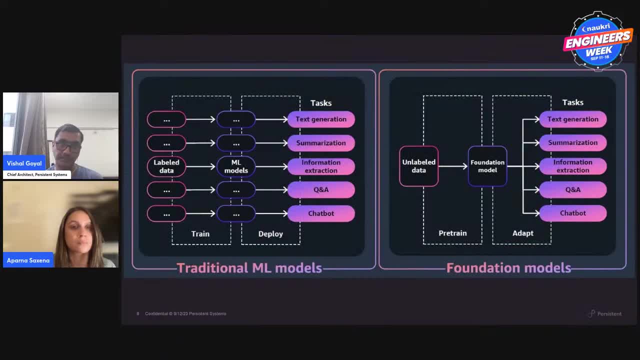 The way you want to do it. This is important for people. What is changed? So, if you see on the left hand side, you have traditional ML model. This is how AI was always being used for many, many years And we could still do whatever we are doing today. 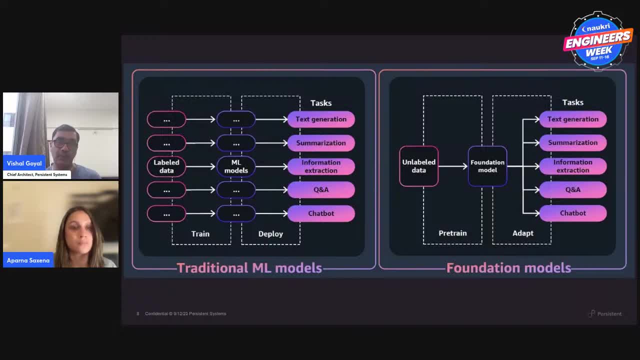 We could do text generation, We could do summarization, We could do sentiment analysis. So, if you see, one of the good use cases was when we give reviews- Google reviews for a hotel or for any Airbnb facility- We could do sentiment analysis to say: is that review positive or negative or neutral? 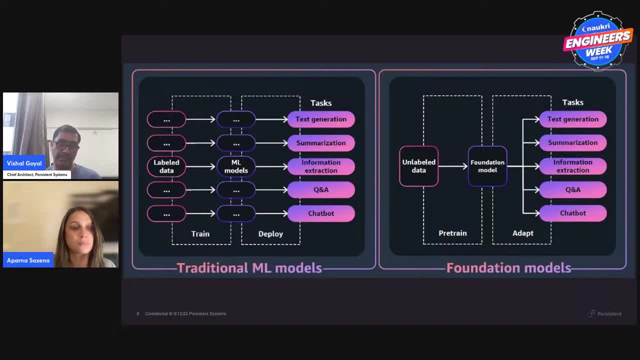 All this was still possible with traditional ML, And that's what a lot of times I get asked: that we could still do all that. We could still have a chatbot, ICICI bank and HDFC bank, and all of them had chatbots. 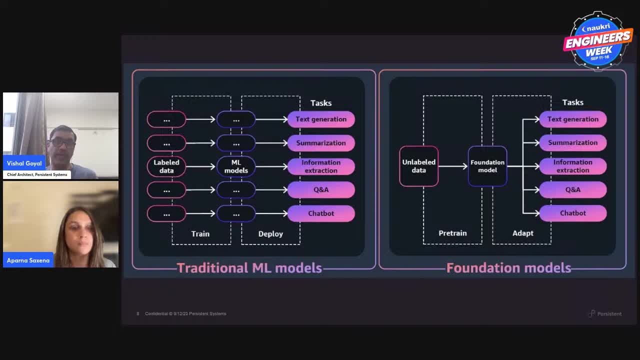 So what has changed? So what has really changed is the way these things work. So if you see, traditionally, as I said, supervised learning, unsupervised learning- you had to train the model and then you had to deploy it at some place for someone else. 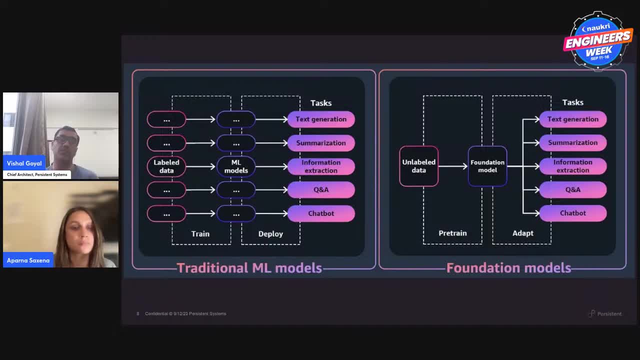 That was the architecture which was being followed till now, But with foundation models, with LLMs and ChatGPD. what has done is these are pre-trained- Pre-trained on large volumes of data, billions of data from Wikipedia, from GitHub, source code repos which are open source, and things like that. 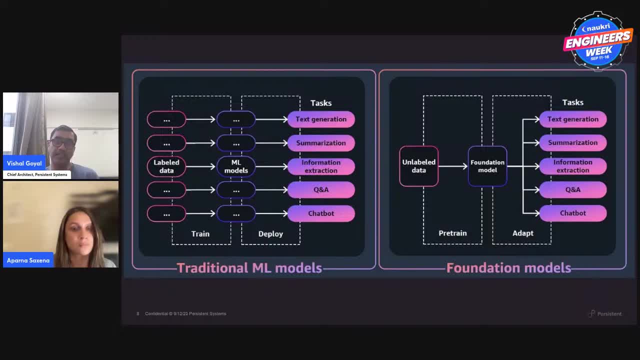 And then what you do is models adapt to it and continue to improve as you talk to them. That's what is called adaptation Deployment. Once you deploy it, it will continue to do what It does today, versus what it does 15 days ago. 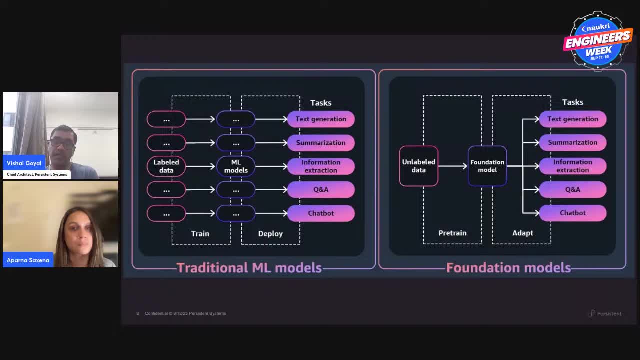 What it will do 20 days from now. But foundation models adapt to whatever you do. whatever you would fine tune whatever you do from tuning, And that's the core difference between it. So no labeling of data has been done, While for training the model, a lot of work has been done. 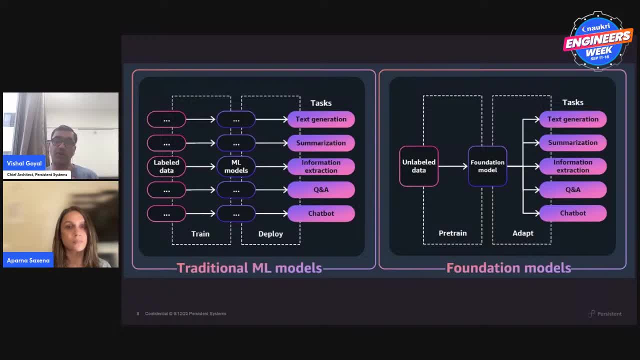 There is a lot of manual effort which is involved to do training and reinforcement learning and all But all that has been done by OpenAI. You don't, You don't, You don't have to do that. But once all that is done, you get a pre-trained model and all you do is use that to write a book, write a story, whatever you want to do. 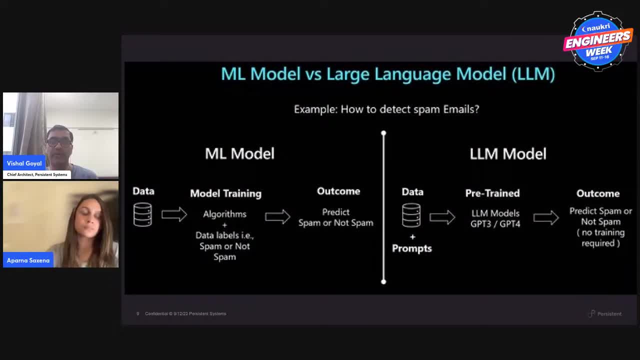 This is one example. So on the left hand side you again have how do I detect spam emails? So you have Gmail which will track whether the email is a spam email and they'll track it to spam. And it basically was a model which was trained and they had labels done: spam or not spam. 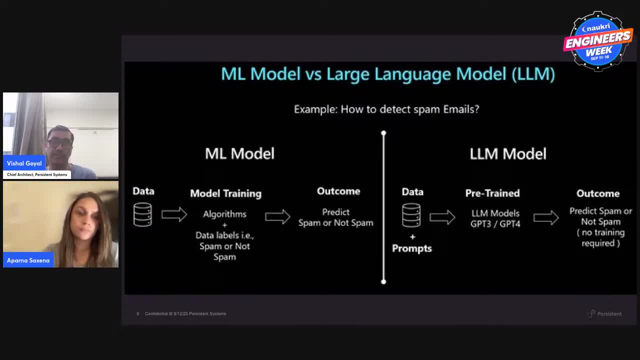 And that's how it would done LLMs. what is happening is it is pre-trained large language models. You don't have to label any data, You don't have to put any algorithms And, based on the prompt, it is basically detecting an outcome, whether it is spam or not spam. 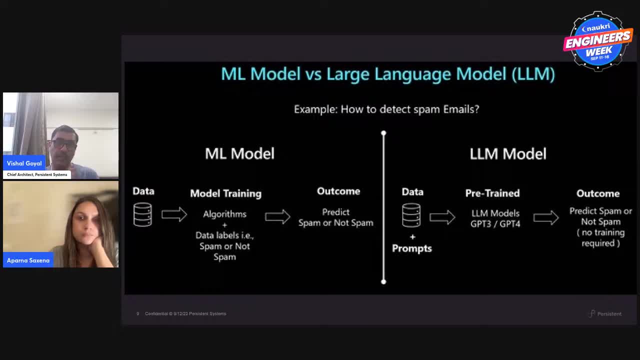 So extremely important aspect is: no training is required to use the bare manila LLMs. Yes, some level of training is required if you want to do a fine tuning, which we will look at in the subsequent slides. A lot of times people ask what is the skills which we should base our training on. 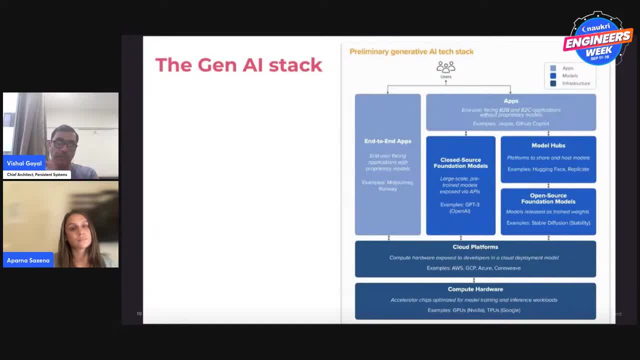 So let's go back to pre-gen AI and we had people writing code who were developers. You had people writing test cases who were testers. You had cloud engineers who would focus on having skills on AWS or Azure or GCP And they'll say: we are cloud architects. 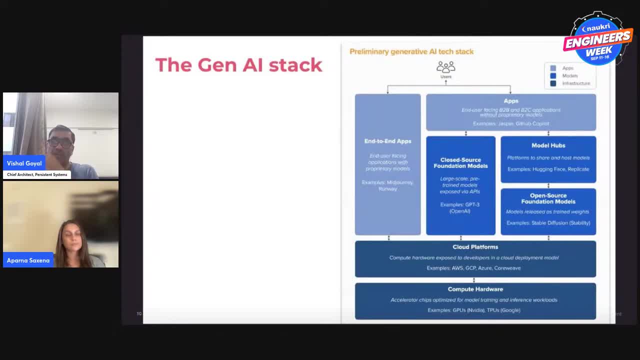 We are certified on cloud. We have done five certifications, and so on. Then you had infra guys who would say: we know how to set up your cloud environment. We are your DevOps guys, whether you want to do it on-prem or cloud. 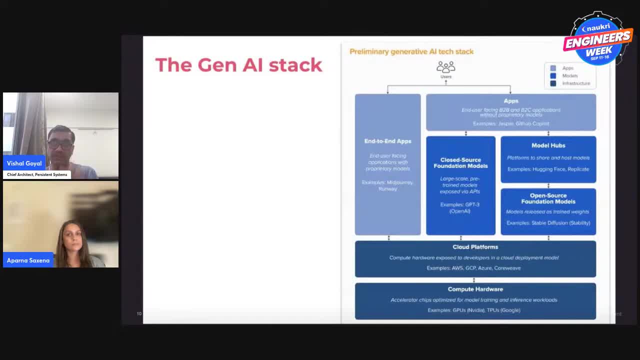 And we know how to set up your environment. We understand which services to use, how to set up your VPNs and networks and things like that. Something very similar has happened with this gen AI tech stack as well. So you have applications, you have models and you have infrastructure. 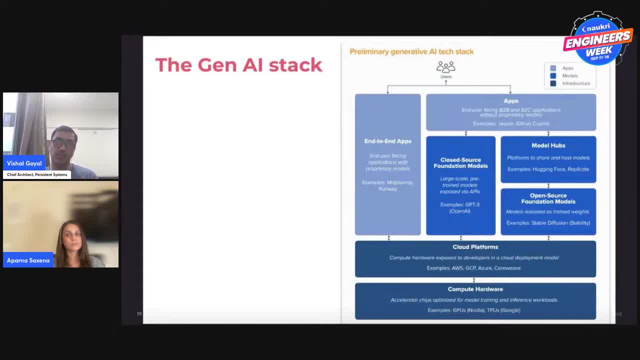 And people who are looking at entering the gen AI space would then pick and choose which area of gen AI stack they want to build their skills on. Not one single person would have skills across this entire stack. So some of you may say: we want to build this entire stack. 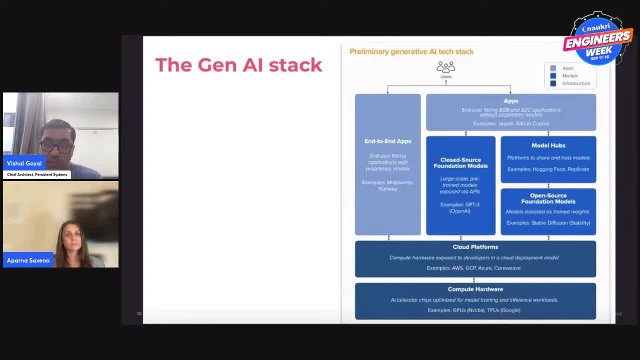 We want to look at the hardware side of it. How does GPUs and TPUs which are used to run these models on? So AWS has their own infrastructure. Similarly, NVIDIA has taken up And you see, Reliance and Tata have just joined partnerships with NVIDIA to use their chips and so on. 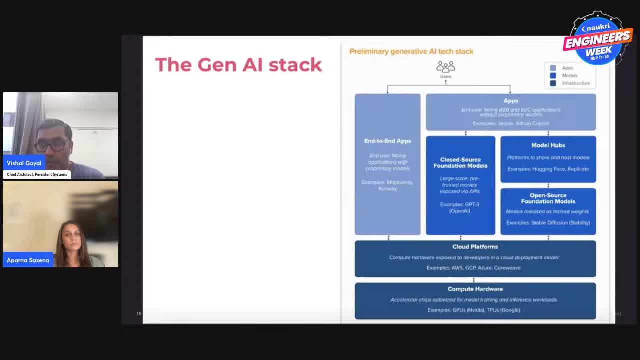 That's one area of the skill set. Second is your cloud platform. So how do you use these cloud platforms? So a lot of people on this call may have skills on cloud already- They may be AWS certified or Azure certified and things- And they may say, yeah, I already know cloud. 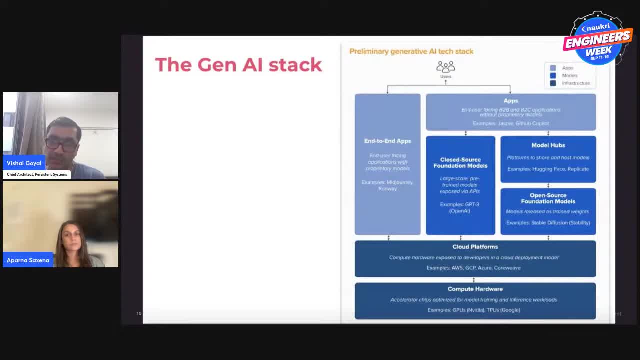 How can I use that skill, which I've already built over the last few years, to really accelerate and come into gen AI? And that's where you have solutions from Azure- You have open AI and you have Azure ML studios. Similarly, from AWS- you have AWS Bedrock and you have AWS SageMaker Jumpstart. 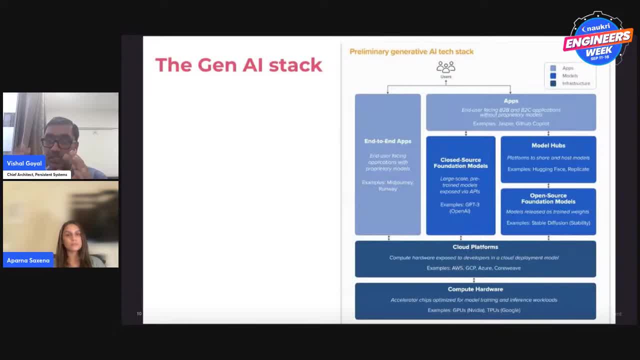 Those people who already have good, strong cloud skills should then get into that space and start understanding this space Right. Then you will have people who would be kind of developers and who would want to know: I'm a developer. I absolutely am not a data scientist. 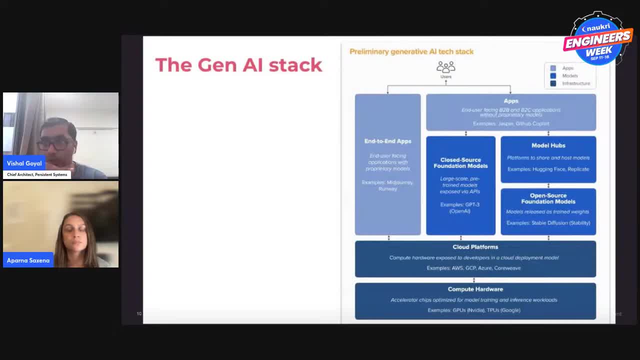 I don't know a lot of machine learning skills and all, And I cannot learn those skills. What is the area which I should then probably look at Right, And that's where the apps piece of area is extremely, very important. So you have solutions from Microsoft like Copilot. 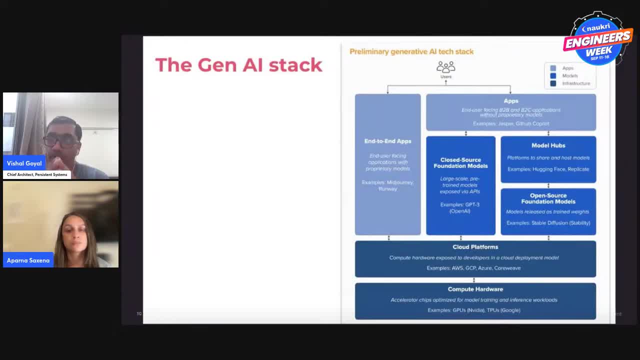 You have CodeWhisperer from AWS. You have Kodi SourceCraft. You, as developers and engineers and testers, should know How do you use this solution to be able to do different stuff in software engineering, Whether it is to write a code fresh greenfield. 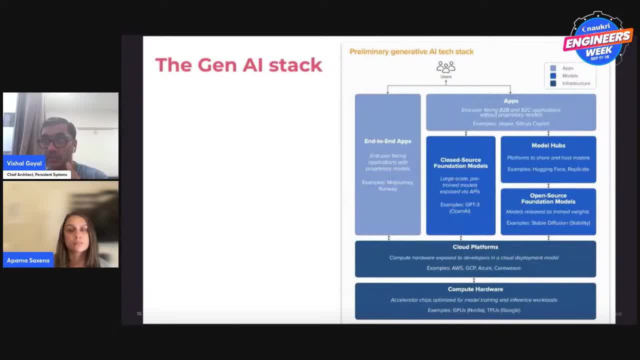 Whether it is to explain an existing code and understand the business logic, Whether it is to be able to convert this code from one programming language to another. That's your core strength: You are able to write code in Java or C-Sharp or React or whatever language you are. 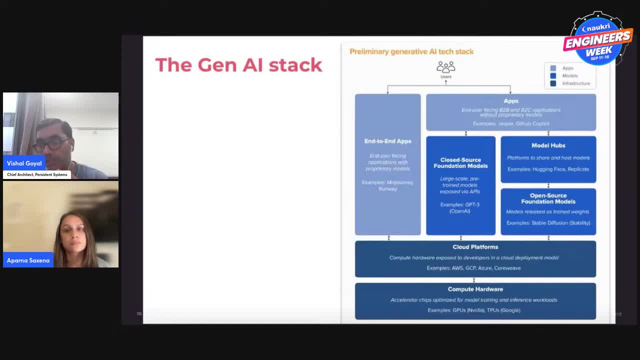 And then you play in that space. You don't get into the below space, which is code, dataset, Data science and things like that, Right. And then there are data science engineers who will say: we want to train these models and make it very tuned with our own customer data. 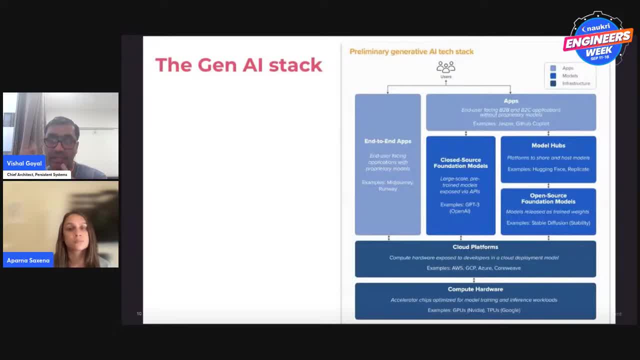 So customer will say we have volumes of data as it is, because that's consumer grade, That's not enterprise grade And we want you to support us to fine tune the model with our own dataset and ensure that we can deploy it in an enterprise. 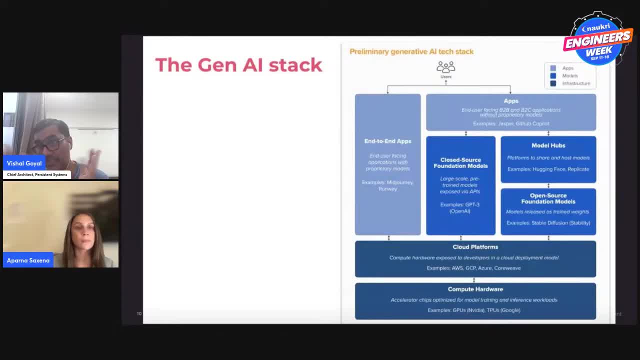 And it only responds to our questions, Right. So, as an example, If I am as persistent, I have HR and I want to deploy a model which will only respond to questions which are HR related Right. When do I get my salary? 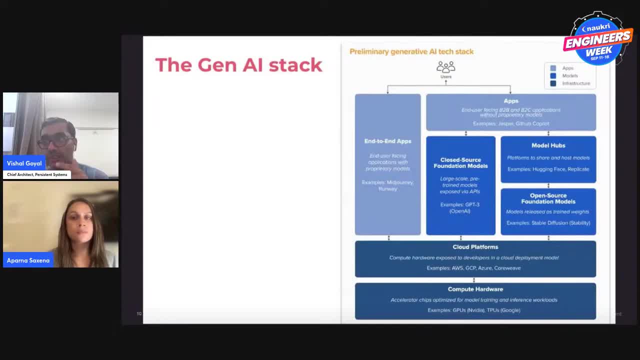 Where do I see this policy and this and that? That's where you will start then training these models. Or you will use a lot of open source foundation models to build very bespoke custom applications, Right? So that's another area. The reason why I wanted to put this slide again is for people on the call. 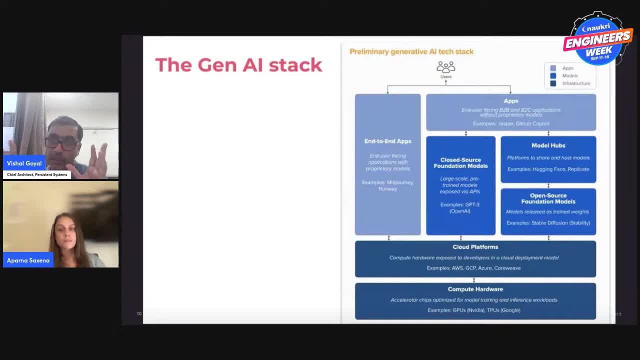 If you are interested, on which area of gen AI should I pick up? because there are too many things. A lot of this is not known to people and people see gen AI as something which is only chat GPT. No, it is not Right. 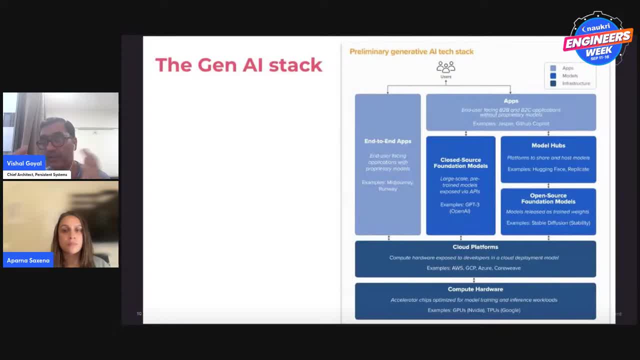 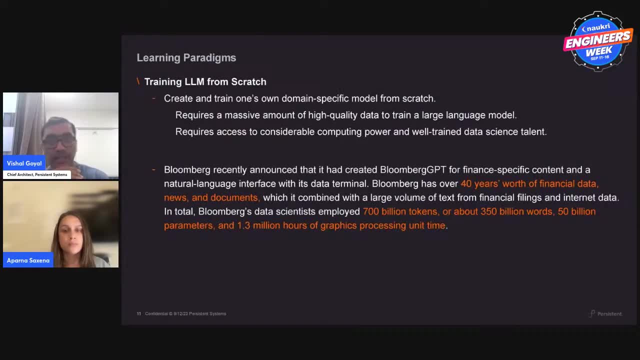 So your core skills which you have built over the last few years as part of the industry, or even if you are fresher, you can pick up what the area of choice for you is and then start looking at it from that angle. Yeah, What I want to do is go to the next section of my presentation and talk to talk about what are the learning paradigms. 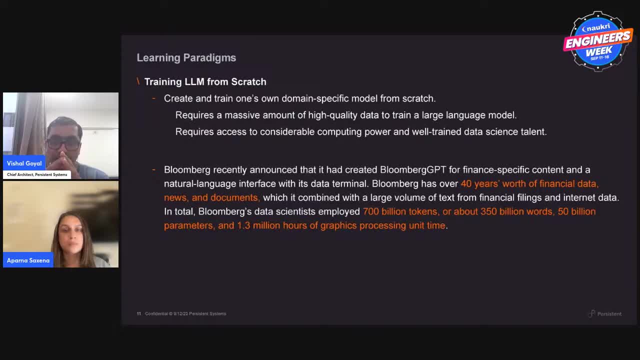 Learning paradigms, which means: do you want to build your own LLM models? So let's say: you have money, you have document, you have the infrastructure and you say: I want to build my own LLM, which is what Meta is doing with LaLama now, which is what OpenAI did with GPT. 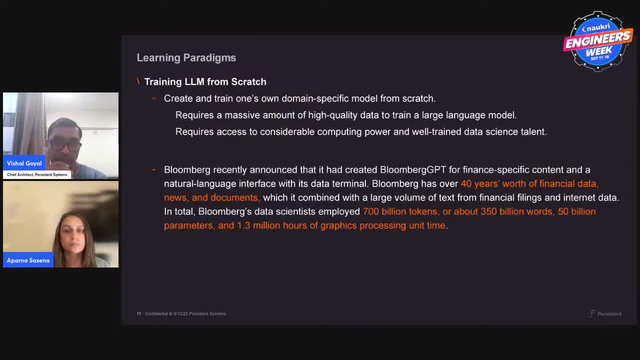 And if you have beans, why not do it Right? So this is what training LLMs from scratch is: You will create your own domain specific models. The challenge with this is, as I mentioned, this requires massive effort, Right. 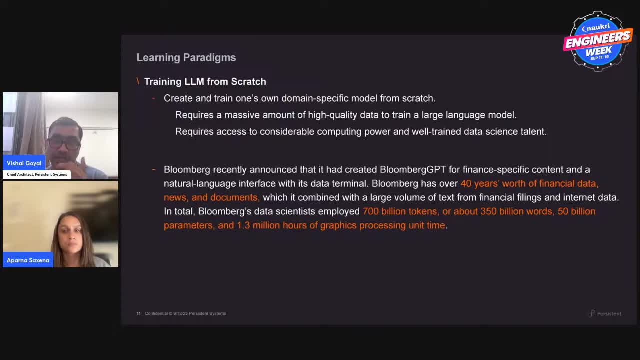 It requires massive amount of high quality data, It needs a lot of computing powers, It needs a lot of data science talent to be able to do that. Now, is that impossible to do? Of course not. Right Bloomberg did it. So Bloomberg picked up the GPT model and that said: we want to train it for financial related data. 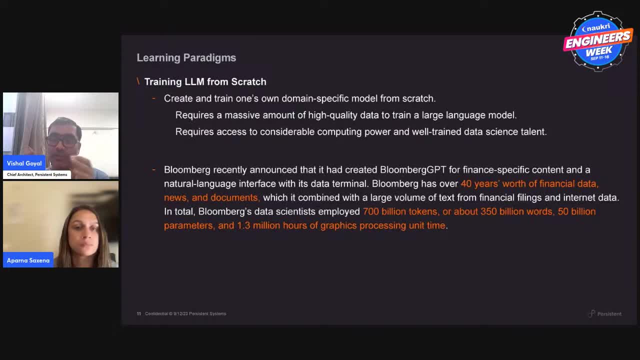 So anyone talks to Bloomberg GPT? it will have a very strong context of financial data And if you see the items highlighted in color, you will see they had 40 years of financial data. They had 1.7 billion tokens employed, 350 billion words, 50 billion parameters and 1.3 million hours of GPU time. 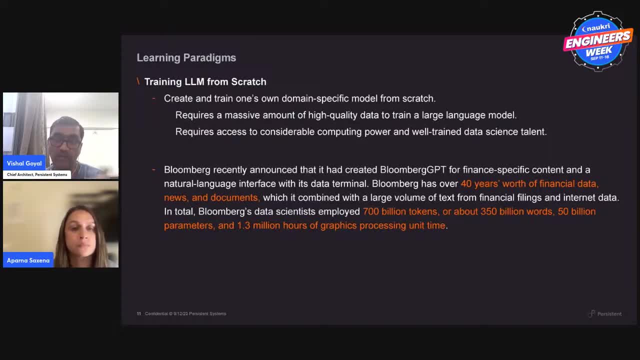 How many people on this planet or how many people on this call would have that kind of resources? Probably not, Right? So is this an area which you should get into Again, not for people like you and me, but for large organizations who have these resources? they can look at this space. 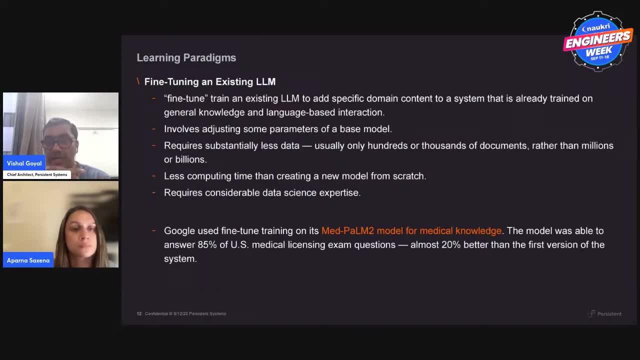 Something which is doable, something which Persistent is looking at. something which a lot of organizations are looking at is this area of looking at LLMs. So you fine tune or train an existing LLM to add specific domain content which is already trained on generic language. 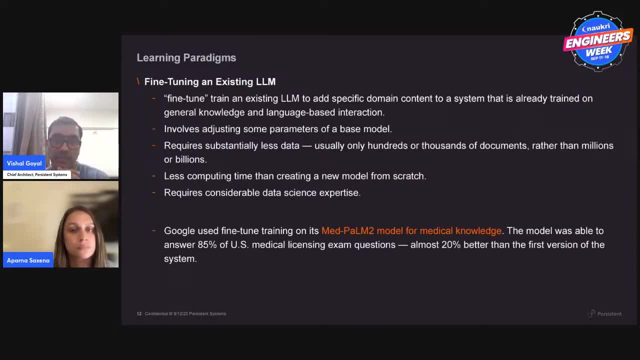 So this means some adjusting of parameters of the base model, substantially less data, but still needs a lot of data science expertise, And that's what Google did. They released a Palm model earlier and then they released a Palm 2 model, which was dedicatedly trained on medical data. 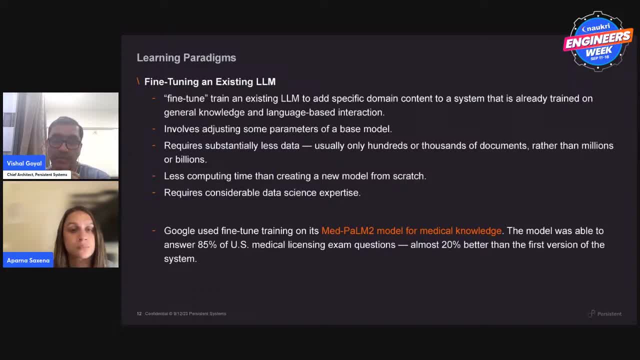 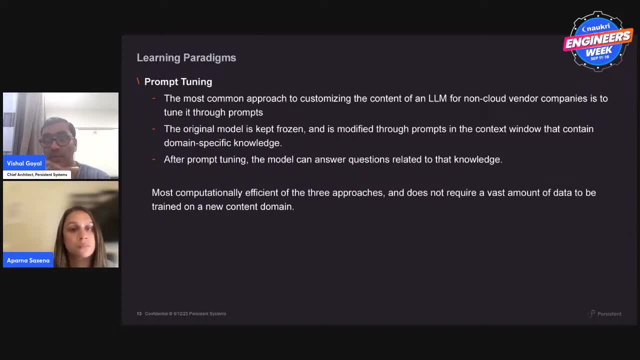 And you see the model here. The model was able to answer 85% of your medical licensing exam questions. Third piece, which is where I do a lot of my work with my team as well, and which is the easiest of the three approaches and most prominent. 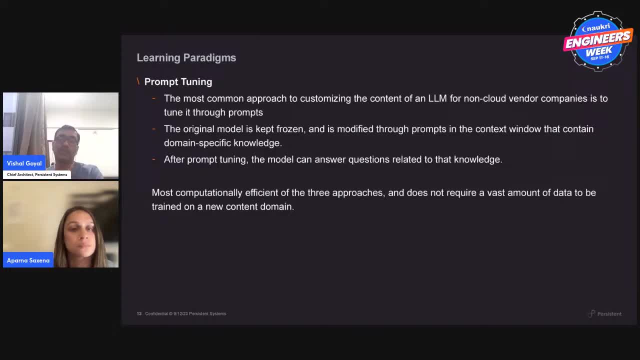 which can do most of the stuff which you want to do without really needing a lot of data science expertise. What it needs is know-how of programming languages to be able to use framework. Langchain is something which is most commonly used. You have semantic kernel as well. 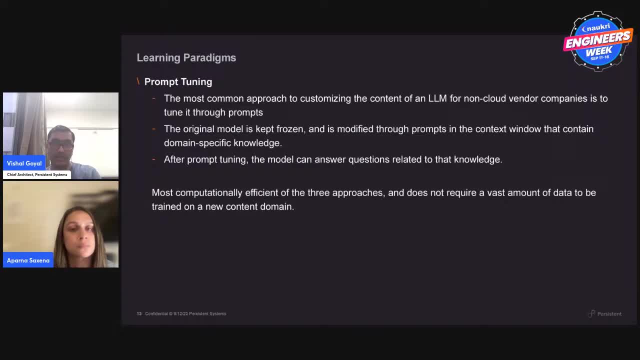 Which is there from Microsoft, now open source. This is something which is doable and reasonable for people to be able to do. So all you do is you are basically tuning the model with your own prompts, with your own content. to a certain extent, 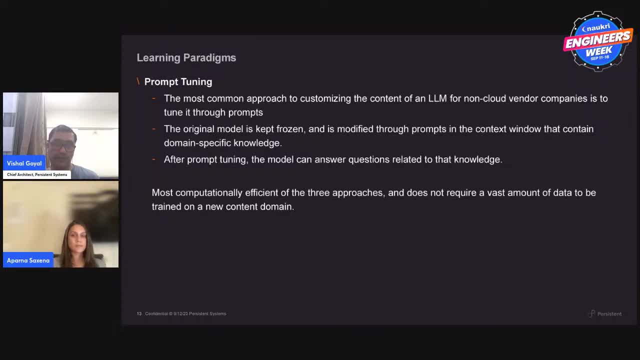 And that's how you are able to train the model, And this is computationally most efficient from the three approaches. Doesn't require vast amount of data, So you will use your own data. So imagine you have your financial reports within your own organization. 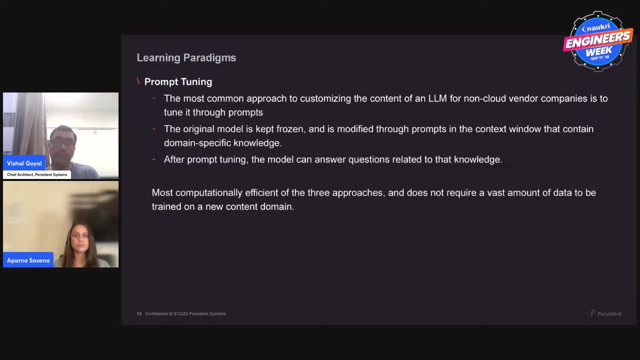 And you wanted to be able to prompt you in a chat GPT And you have your own version of GPT deployed, While you would still use something like OpenAI to create embeddings and vector database, But you would ask questions and the responses would come based on your own data set. 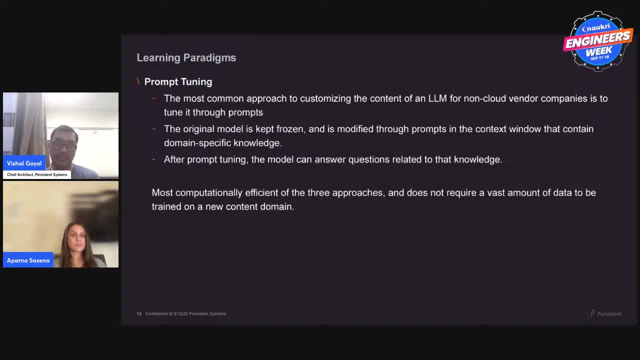 Not on data, which is there globally available in chat. So that's where three important areas in terms of understanding how you can use LLMs: You build your own scratch LLMs from scratch. You build fine-tuned LLMs. You will fine-tune those LLMs with vast amount of data to make it domain specific. 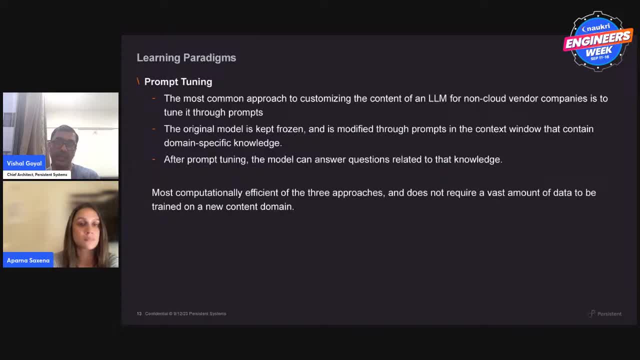 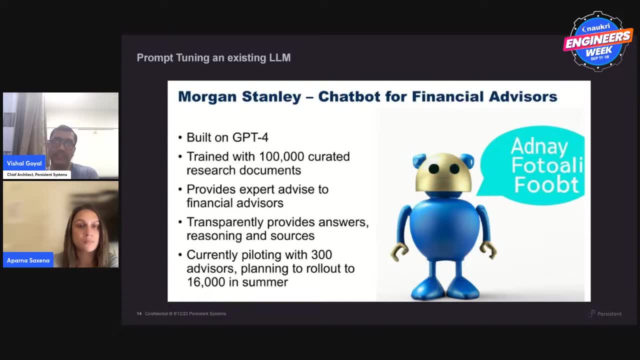 Or you do prompt tuning with smaller data set But still restricted to your own data when you talk to it. Example of prompt tuning: Morgan Stanley. So they created a chatbot for financial advisors. They used GPT-4 based model, Trained it with kind of 100,000 records for search documents. 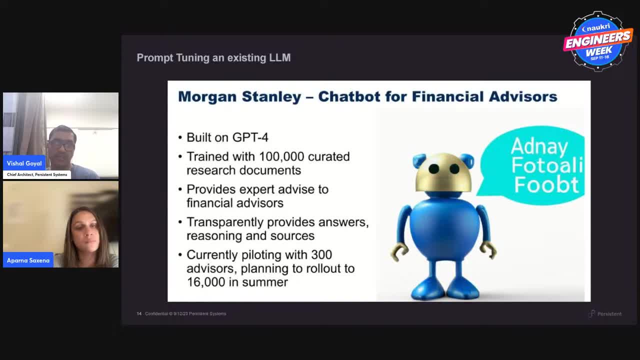 And then it is able to provide expert advice to financial advisors Right And piloting it already with 300 advisors Rolling it out to 16,000 people. So I gave you three examples in each of the three areas: The large, the scratch models, which is already available and known to people. 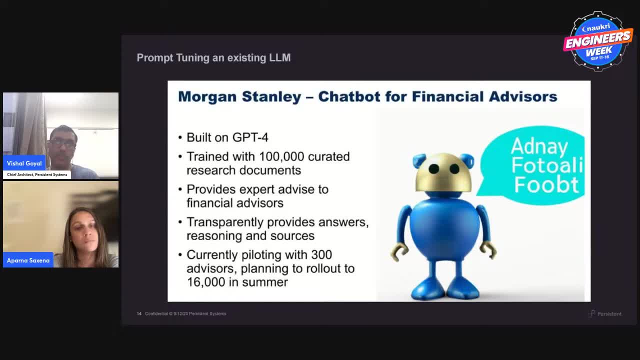 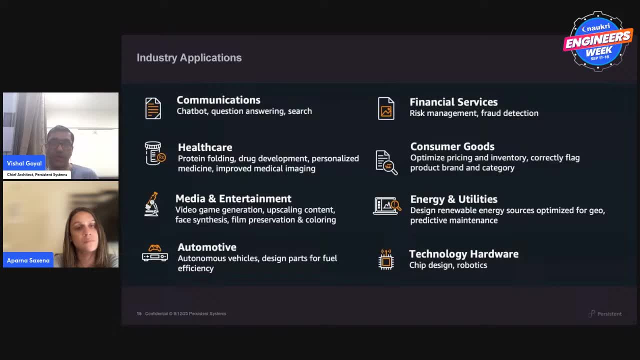 The fine-tuning, which is what was done, And then you have the prompt tuning, which Morgan Stanley did. Again, this is not just related to software engineering, So a lot of these industries have started using these technology of J&AI for solving different problems. 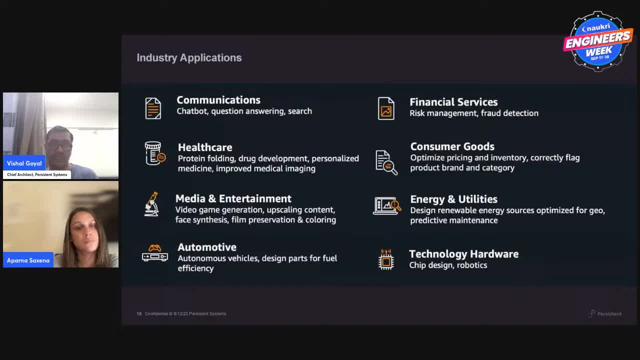 You see communication industries, obviously around chatbot and question answering, But healthcare has started doing a lot of this work around development. We as Persistent are engaged, So healthcare and life sciences is an important area for Persistent And we do a lot of work with the global healthcare customers across the globe. 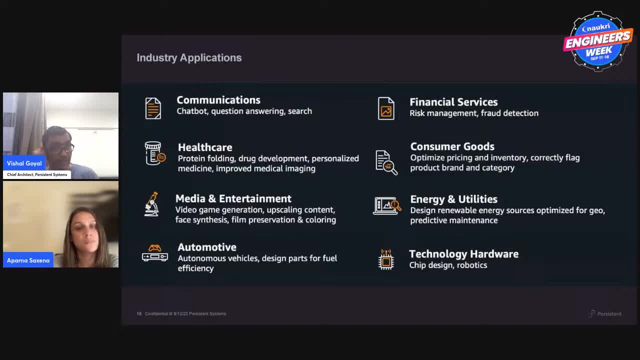 And we have been talking to them on how J&AI can be used Again, media and entertainment. Content creation is a very important area which is known to everyone mostly, So you and me can also create content very easily. If I wanted to write a story today, I can give it a simple prompt saying: 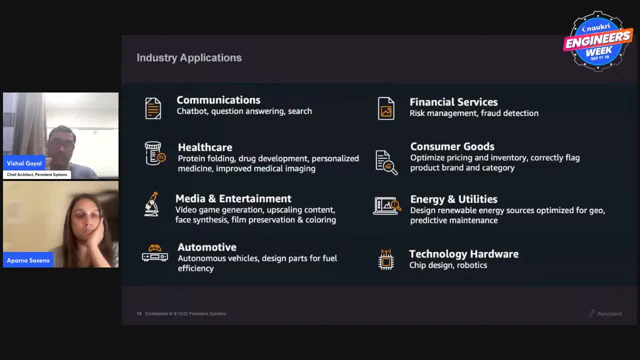 I want you to write a story about something And you describe a scenario like you define a user story And it will generate massive beautiful content And if you were to use some of these solutions like mid-journey and others, you can actually create a film with video content and things like that. 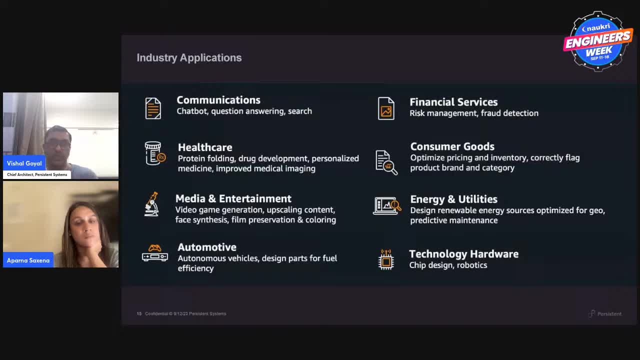 So, as I said, it is not just text. You can use it for multimodal text, images and videos and things like that. Financial- we already spoke about Bloomberg GPT, So a lot of companies like MasterCard and Visa would start looking at using 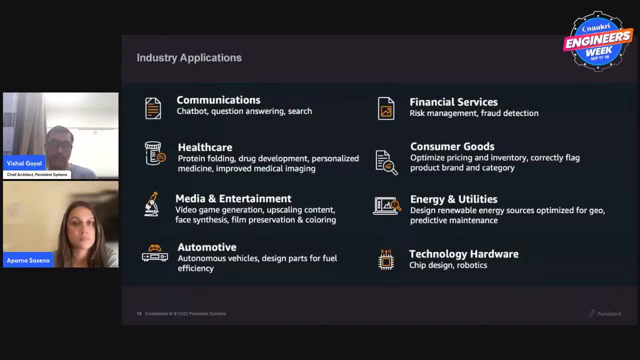 generative AI for doing fraud detection and risk management. Again, very important for people to know: all this was still being done. As you saw, the traditional ML models would still be able to help you do fraud detection. Now J&AI is obviously escalating it and taking it to the very next level. 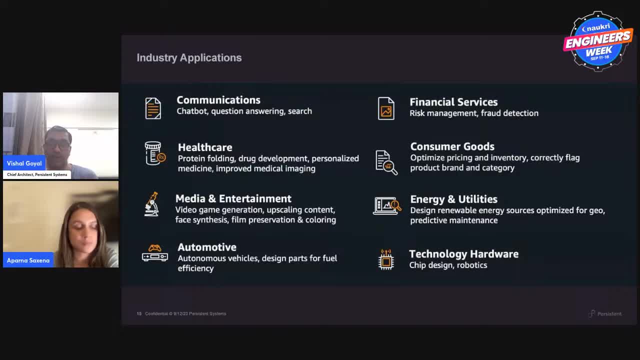 wherein it is pre-trained. It has large volume of data, It has context there And all you are doing is tuning in top of it. So a lot of use cases across different industries. This is just a sample But, as I said, we have spoken to more than 100 plus customers around J&AI. 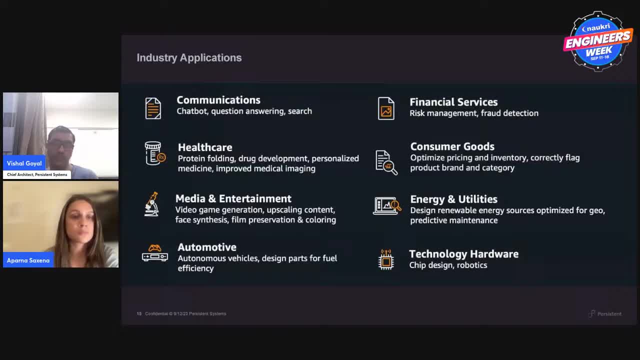 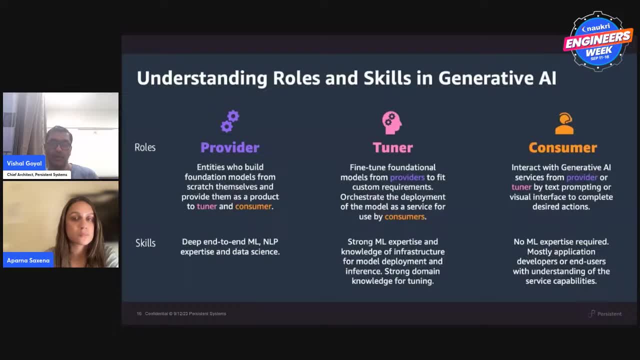 in the last few months And we have seen very different use cases coming in from different industries. Again, an important slide for people on this call on what do we do, what kind of skills we build, And I touched upon this in my J&AI. 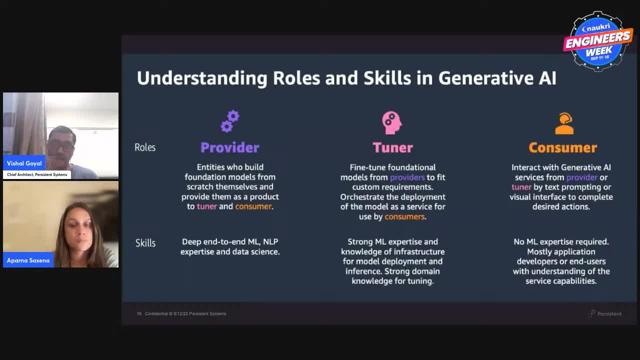 I talked in terms of where you should play, But again, you see, different organizations would play different roles. So there will be providers who would look at a product and creating a LLM model, And they will build foundation models from scratch, like I showed you in the earlier slides. 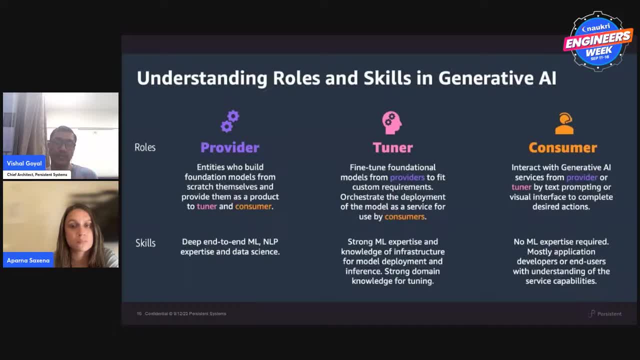 And they are the providers. They would need deep end-to-end ML skills, NLP skills, data science skills. They would have hardcore data science engineers who would start building these models, Something like GPT. So if we had to build something like GPT from scratch, 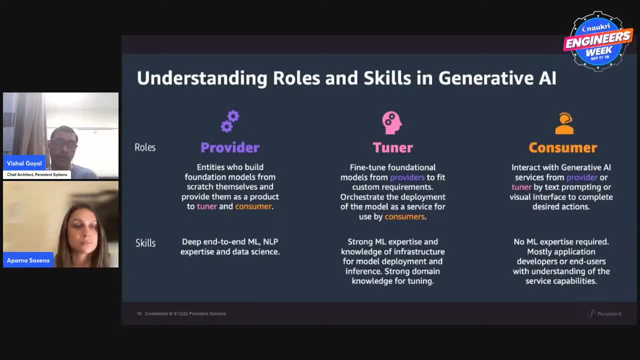 that's what these providers are doing. AWS has built their Titan model, Microsoft would build something else, Or they will use OpenAI. Meta has built LLM, And then you have companies in UAE and others building a lot of these models, And then you have Tuner. 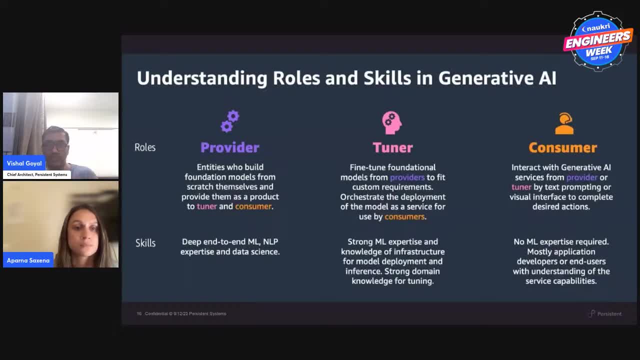 These are the organizations who will say: we will not build something which providers are doing, But we will use what providers have given to us. So we will use GPT 3.5.4.. We will use LLM model. We will use Titan models. 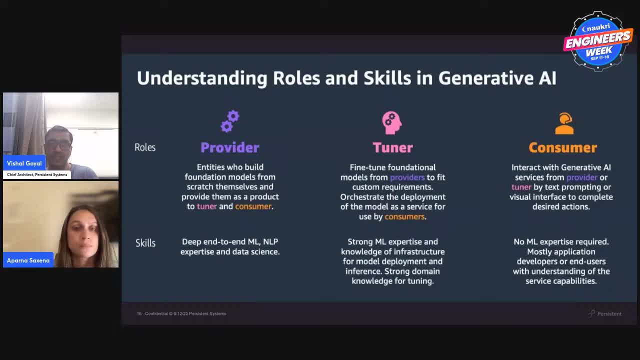 And we will fine-tune them and create our own applications for people to consume. So they would still be in the business of creating something for B2B or B2C, But they will then fine-tune what has been given by providers. 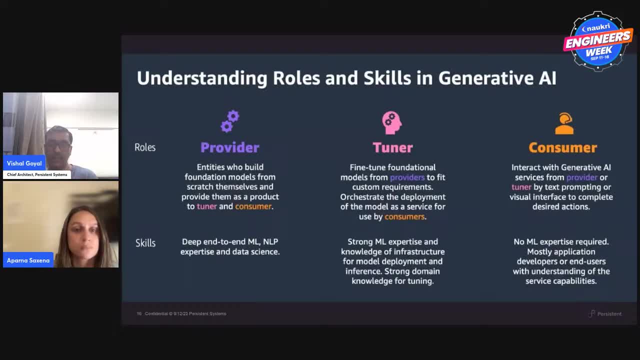 They would still need ML expertise, but not as deep as the providers. And then you have consumers, which is what a lot of people would do. A lot of organizations will do Saying, guys, we will not look at provider and tuner scenarios, but we will interact with the GenAI. 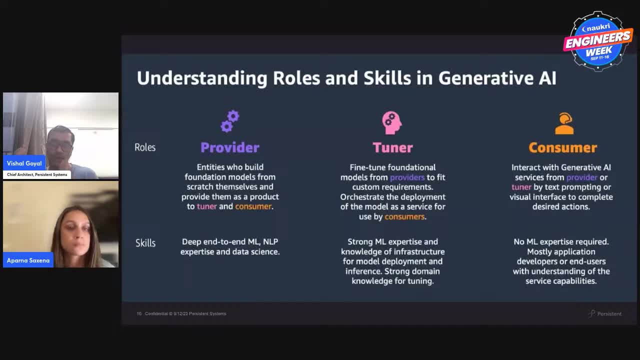 whether using a chat interface or using OpenAI calls. So a lot of this work on consumer space is being done using either the chat GPT 4.0 commercial version, which has an API available as well, or as your OpenAI or the OpenAI APIs directly. 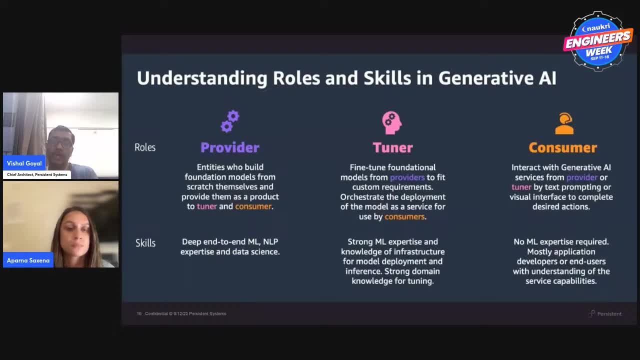 So all these are commercial offerings, then, And they would have security inbuilt as part of this. They will have data privacy, They will have data protection, that they will not use your data to train the existing models. A lot of work today by organizations and enterprises is being done in this space of consumer. 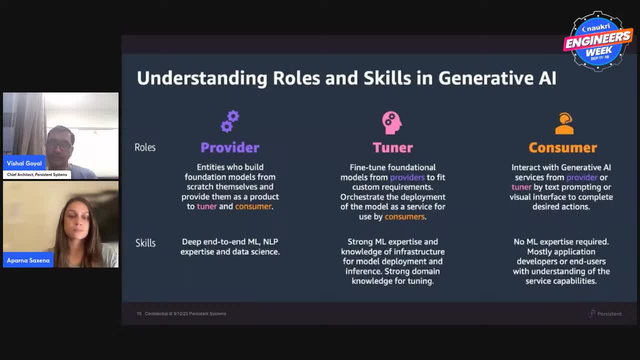 where you use what provider and tuner is giving it and then you are prompt tuning it, And I believe a lot of people on this call should focus on building their skills around this space today, While people who come with the AI ML expertise or people who are doing their engineering. 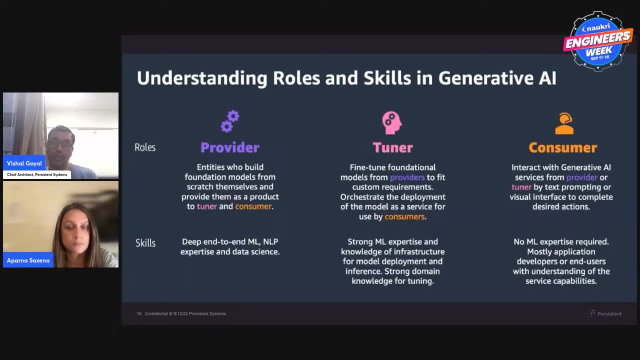 and they are in third or final year engineering and they are doing a course on AI and deep data science, and all could also look at something around tuner. I don't think so. provider is an area which a lot of you people would want to get into. 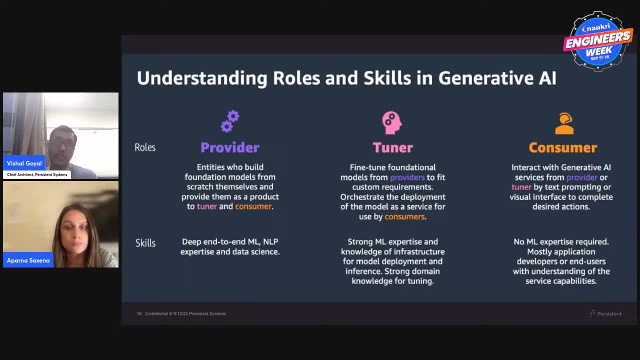 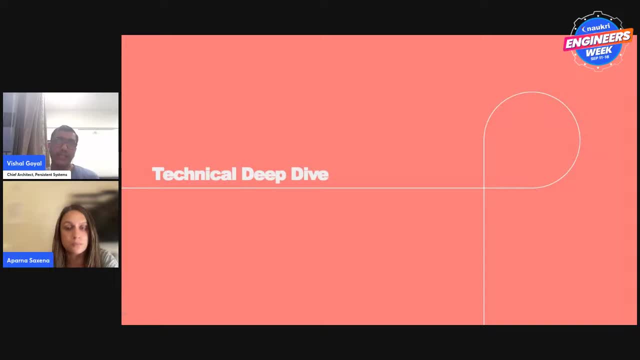 Unless you then join an organization, build your skills and then they are working on that space. We'll do a little technical deep dive now. This is the third section of my deck where we'll talk about little important skills which people need to build. 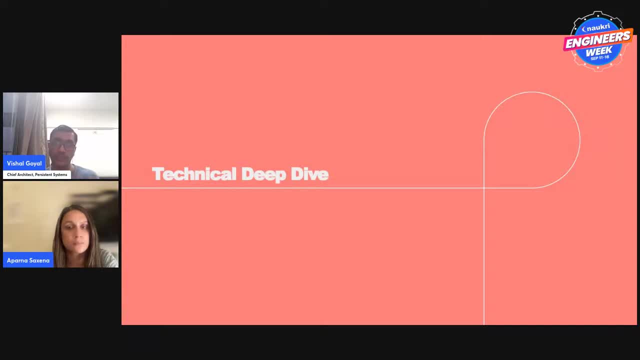 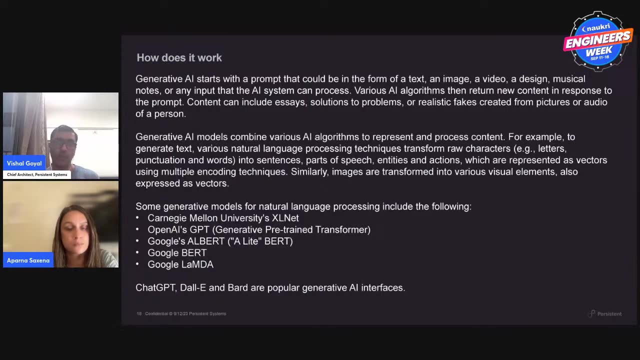 important terms which people need to know to be able to get into GenAI space, especially if you are trying to even understand what GenAI does behind the scenes. So we spoke about a little bit. it combines various AI algorithms to present and process the content. 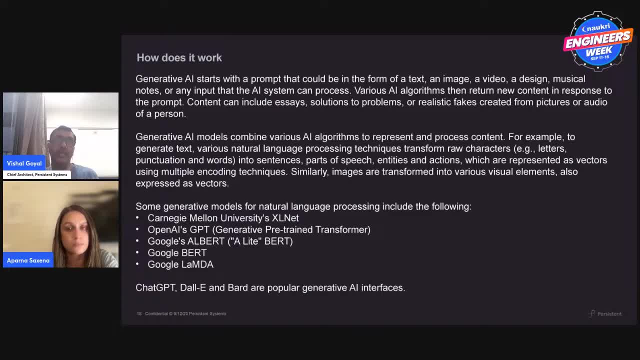 You can give it an entire book. So you have models like Anthropic Cloud2 API which can take 100,000 tokens. now, So GPT-4 can only accept 32,000 tokens, But something like Anthropic Cloud2 API can accept 100,000 tokens. 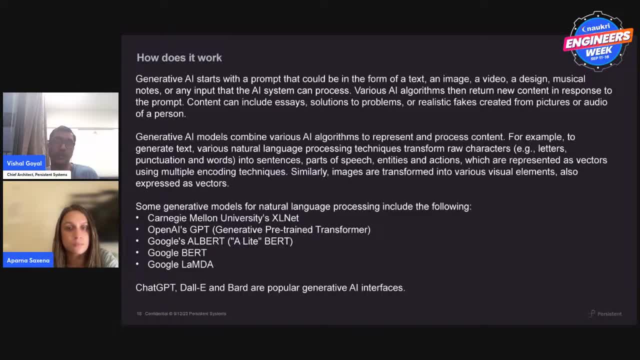 So imagine the power of using a model like that. So you can do a lot of stuff. And that's where these models are available. You had BERT, which came in many, many years ago, But you have Lambda and others. These are models. 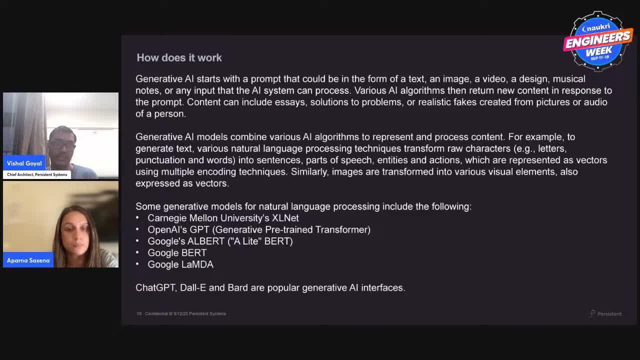 And on top of these models you have GenAI interfaces. As I said, BART from Google is open source, free to use. ChatGPT from OpenAI is open source, free to use with 3.1. And then you have DLA-E and DLA-2 as well. 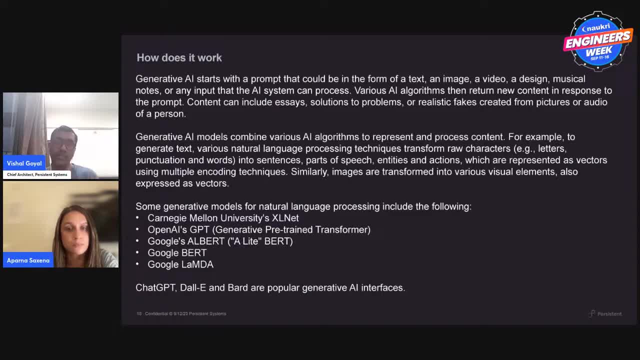 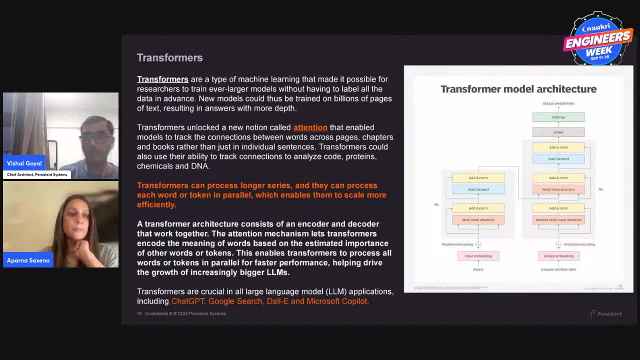 where you can generate images. That's how the things work, But what works behind the scenes is a couple of important things: Transformer model architecture. So people who want to get a little deeper should understand what transformers are. what do they do, how do they work. 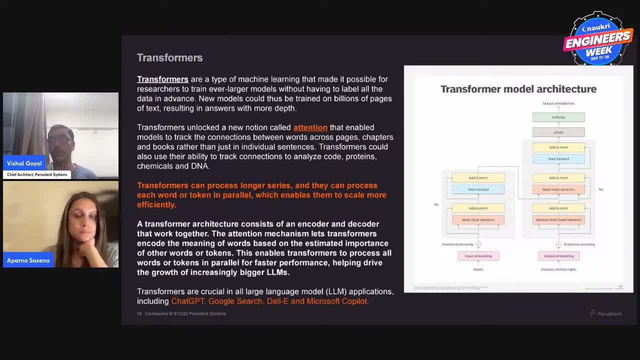 They have something called attention And that's where the conversation happens. So when you write a first prompt and you get a response, what it is doing behind the scenes is there is attention which is happening. So it is basically paying attention to what you said earlier. 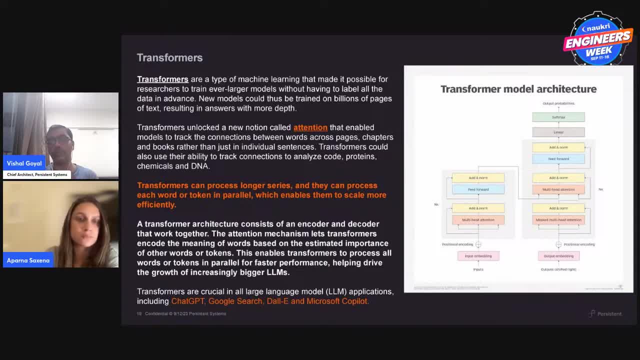 And then when you're saying now, it is basically putting a context to it. And that's where it says that transformers can process very long series And they can process each word or token in parallel, which enables them to scale more efficiently. And all your large language models today. 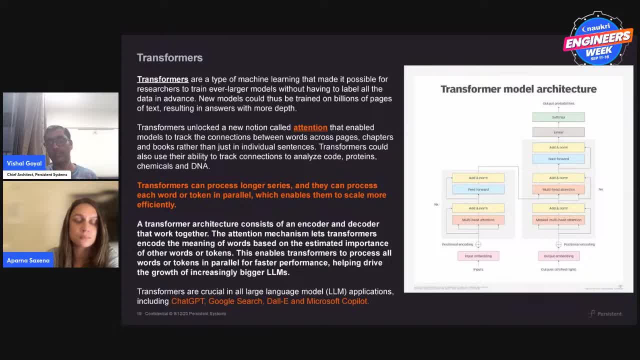 use this concept of transformers. So ChatGPT, Google Search, DALLE, even Google Search, which was there before Jenea as well, would use something like this as an architecture. So people who want to get a little deeper, they should start getting into this. 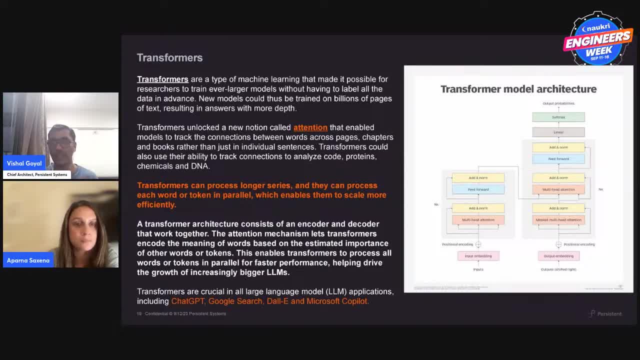 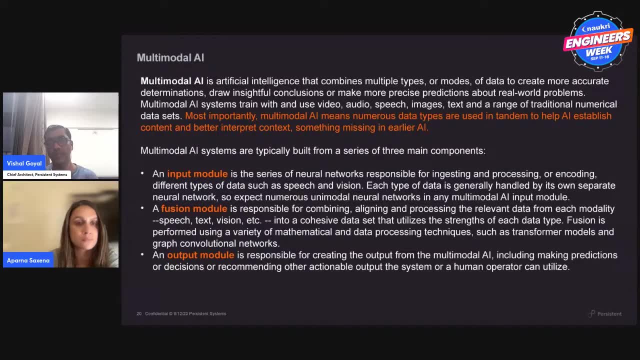 There are a lot of research papers available on transformers and how the architecture works. You can start getting into a little bit more deeper. Again an important concept, So a very big difference between GPT 3.5 and GPT 4.. 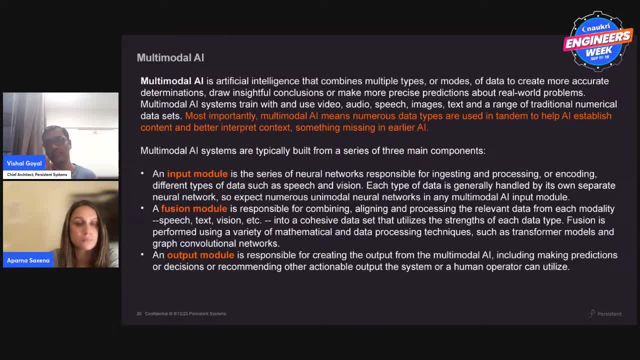 3.5 was text to text, You would send a text. It will respond with a text. GPT 4 actually became multi-model So you can actually get an output which you can have an image. You can give it an image. 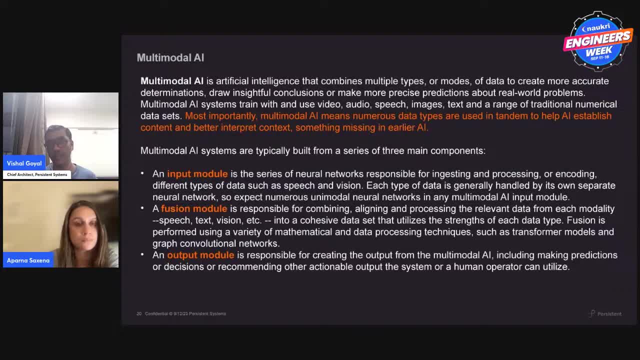 It can process an image. You can give it a video. It can process a video. You can ask it to create a PPT based on your input And it will create a PowerPoint presentation which you can then download. In fact, a lot of people have started using GPT 4. 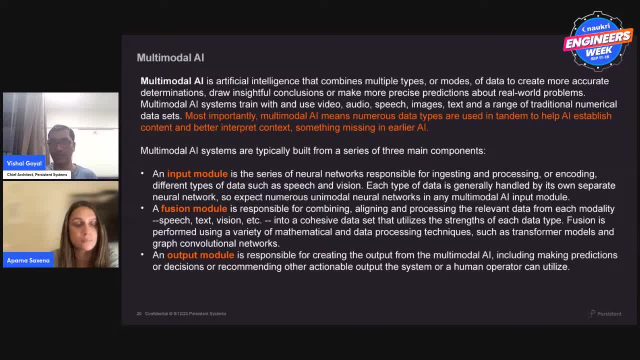 to create a PowerPoint presentation for an executive meeting to say: hey guys, I want you to create a PPT, Four slides, Each slide. First slide should have this. Second slide should have this. Third slide should have this. And what ChatGPT 4 is able to do is really create that presentation. 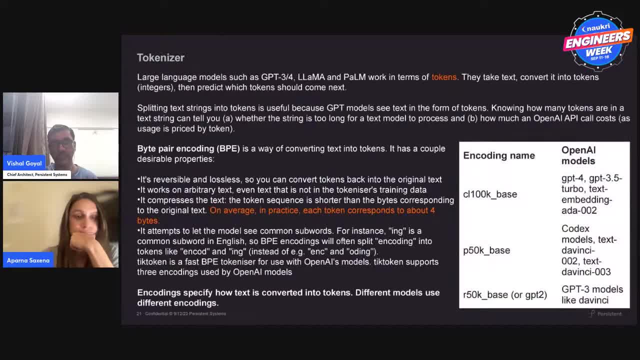 and give it back to you Tokenizer. Very simple. So when you write a sentence today that my name is Vishal Goyal, it basically has certain words: My name is Vishal and Goyal. While you look at the sentence: 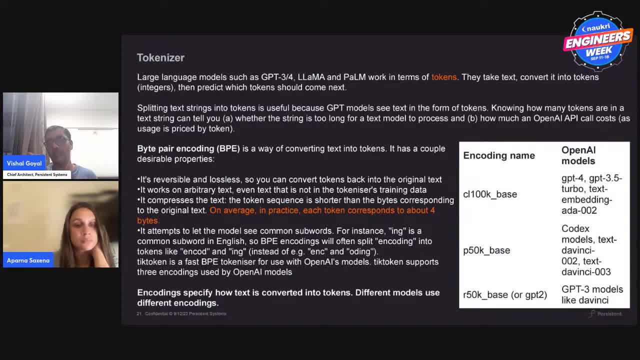 each of them is basically a word And each of these words can mean a very different meaning depending on the context. So, if I use the word bank, bank can either mean a bank close to a river, or a bank can mean the financial bank where you deposit money. 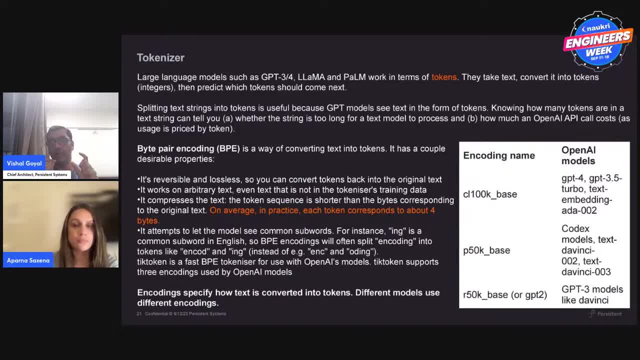 So what is very important for Gen AI to know is: in which context are you using the word bank? Otherwise it will give a very absurd response to you. While you are talking about bank in the context of financial industry, it might give you a response: bank in the context of river. 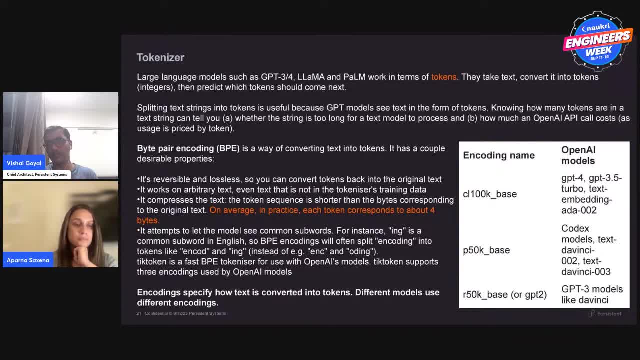 And how this entire thing is work, how these pre-training of the models work is all about tokenizer, And even if you were to do a prompt tuning, you should know the concept of tokenizer. You can use a lot of different tokenizers, while longchains and all these things will have different tokenizers available. 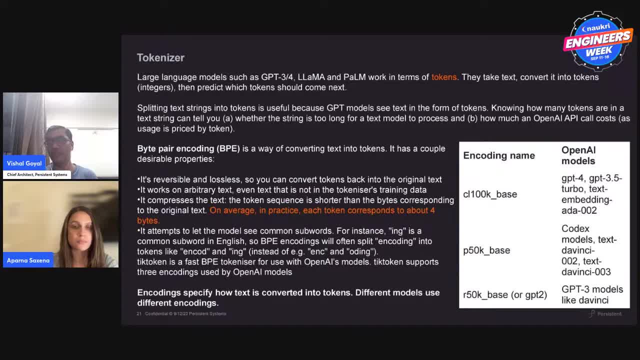 And you see a table on the right where it says there are three different encodings which you can use and the model which it supports. One of the important tokenizers which is used across is BPE, And this is something again people should know to a certain extent. 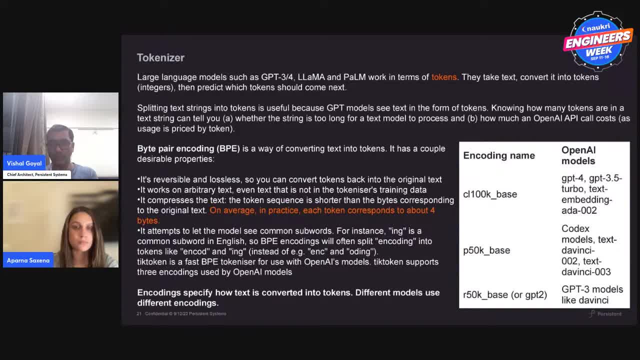 respective of which area of the Gen AI you are looking at. But if you are getting into the Gen AI space, people should understand what encoding is, what coding is and how tokenizers work. So byte pair encoding is is a very important commonly used tokenization algorithm. 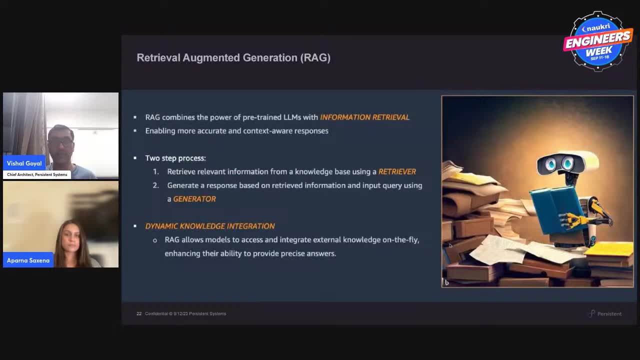 Again, a very important concept which is used in prompt tuning is retrieval augmented generation, And that's how you basically use your pre-trained models to be able to retrieve information based on your own data, which is not large data but small data, And that's how this concept of retrieval augmented generation is. 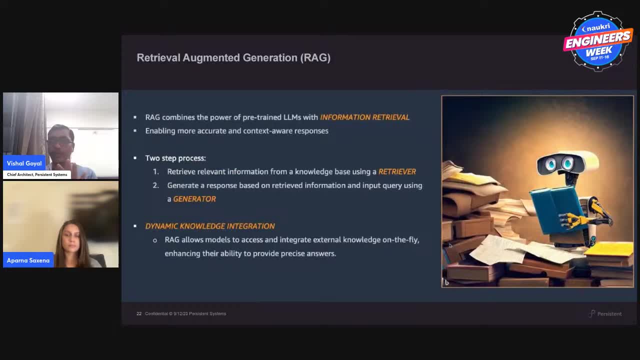 Now, this itself is like a separate discussion and a topic. What I wanted to do on this call is to be able to tell people that this is an important area. You should know what this is. You should be able to use these skills when you use open-source frameworks like LanChain and others. 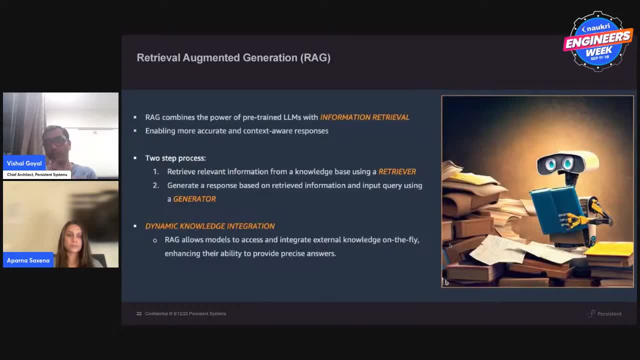 and be able to fine-tune or prompt-tune your models or prompt-tune your applications based on something like this. So, as it says, it's a two-step process: It uses a knowledge base using a retriever and it generates a response based on that retrieved information. 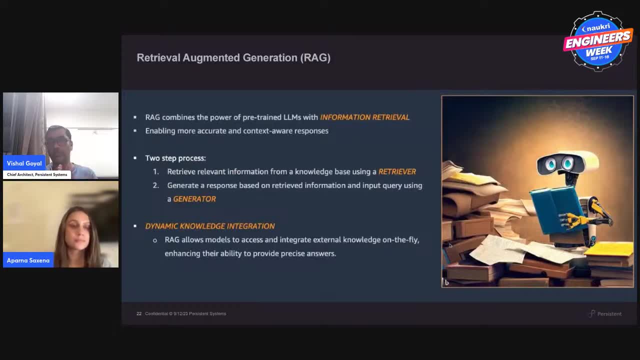 and input query using a generator. So it uses the input query and it uses the relevant information which you have fed into the existing LNs, and then it is able to retrieve and give that response back to you, And this is an extremely important skill for people to know. 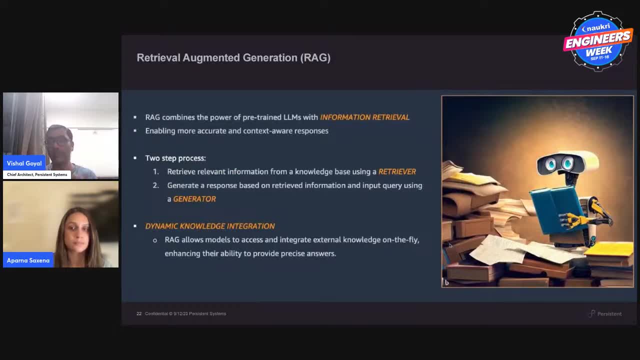 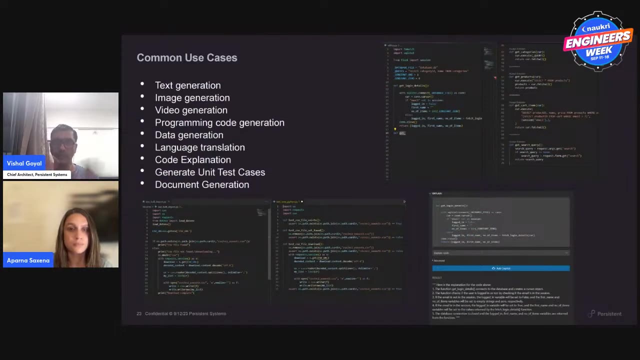 even though you may use standard IDE solutions. But at some point in time you will get out of IDEs and you will start doing something more than just using IDE solutions and app solutions, And this is an important skill for people to develop. Again, some of the common use cases: 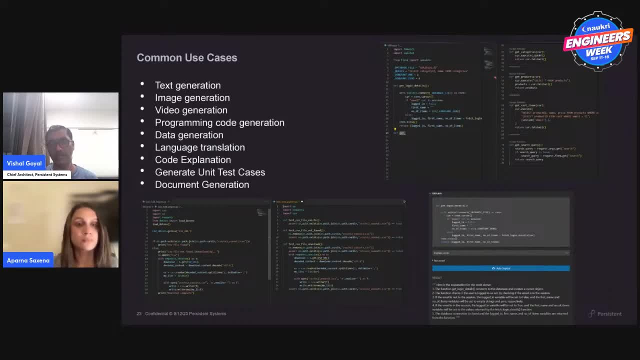 and some of these are based on the work which me and my team does. You have different screenshots, and screenshots are not important and relevant for people to look at. But what is important is you can do a lot of stuff, and we'll talk about the art of possible in my next section of this session. 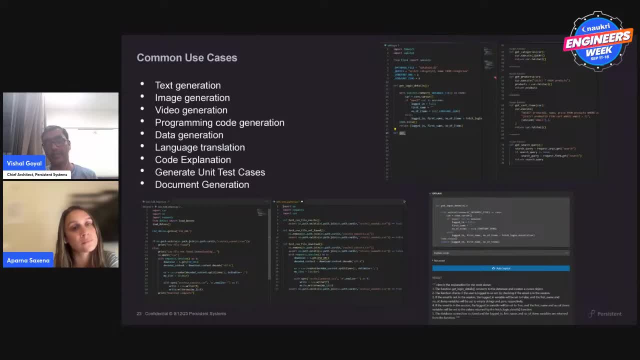 But you can do text generation, You can generate image, You can generate an entire code, which is what we will look at in detail. You can do a language translation span from Spanish to English, English to French and so on. You can explain a code. 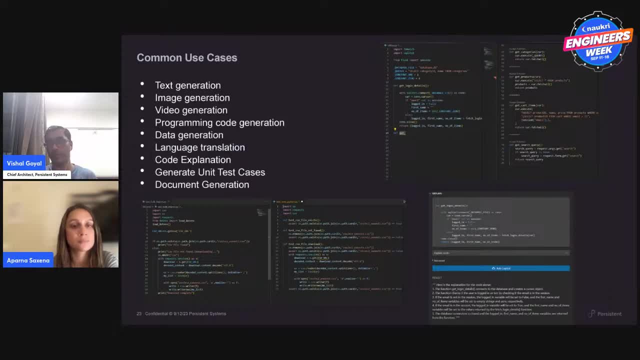 generate unit test cases, even generate a document for your code. So if you had, let's say, millions of lines of code written over a period of time, no documentation exists for it. how do you then create a documentation out of it and keep that document updated? 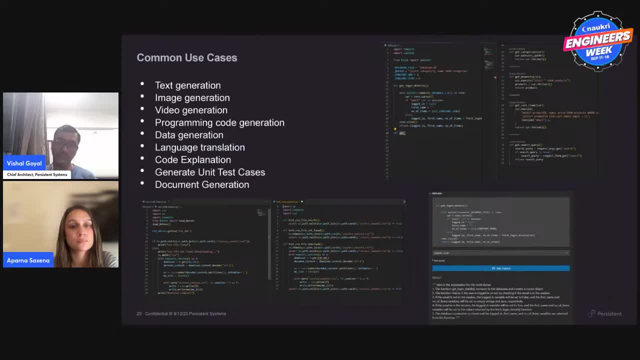 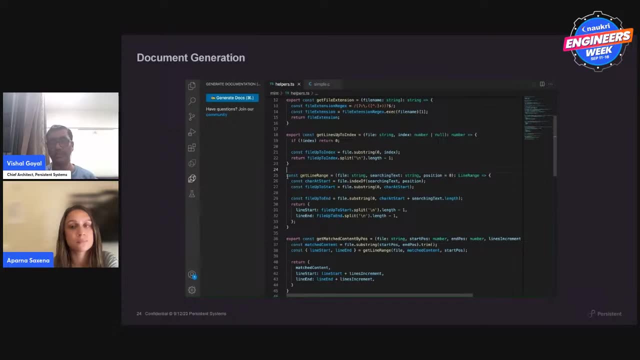 is something which has been possible with the likes of Jenea, And this is just an image of how document generation works. So you have a code and you have tools available. You see on the top left here, you see: generate code here. 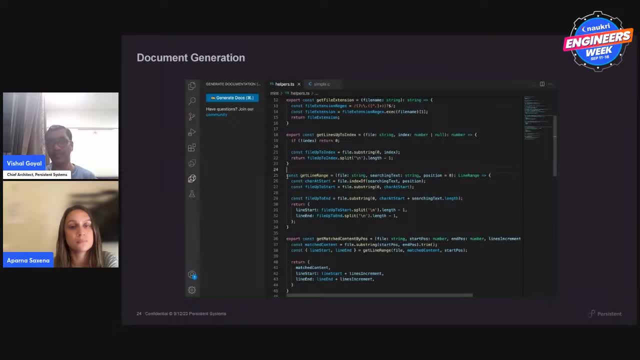 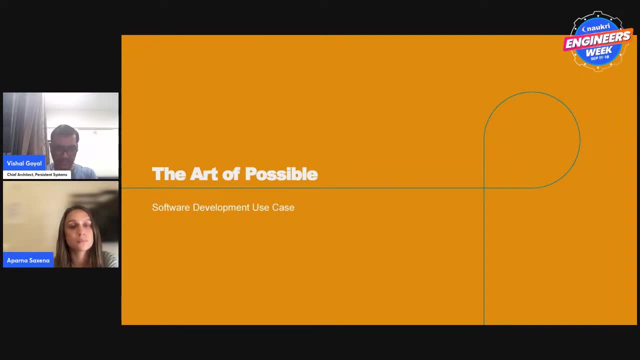 and that's how you can do that: using the ID itself, if you wanted to do it within an ID. Now I'll come to the core, which is the next section, which is the art of possible, which is potentially why all of you are here on. 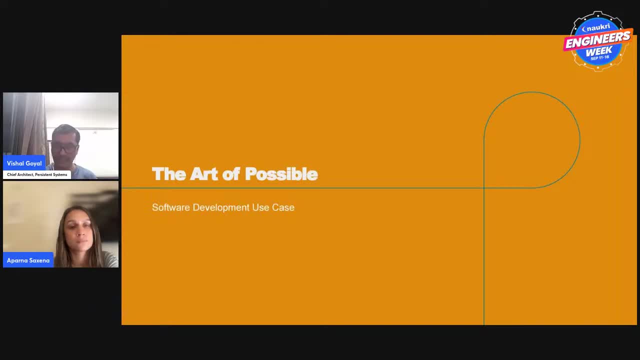 what's possible to be done using software development. Is it just writing a code, Or is it writing unit test cases, Or it can do much more than that, And that's what a lot of work which me and my team have been doing. 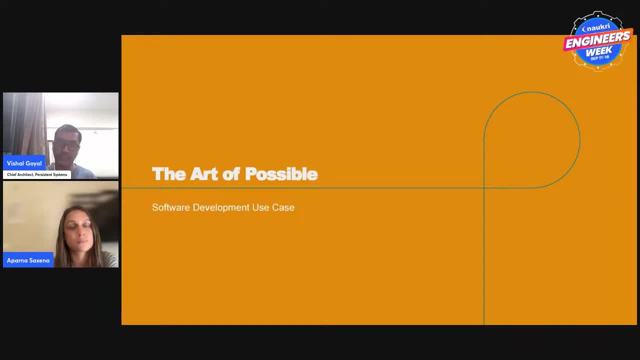 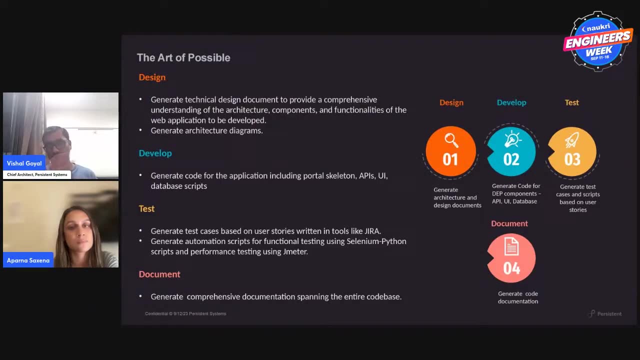 a lot of these discussions- which we have been doing with the customers as well- that do you use Jenea for just writing the code or do much more than that? So this is typical SDLC cycle. You will have a design team. 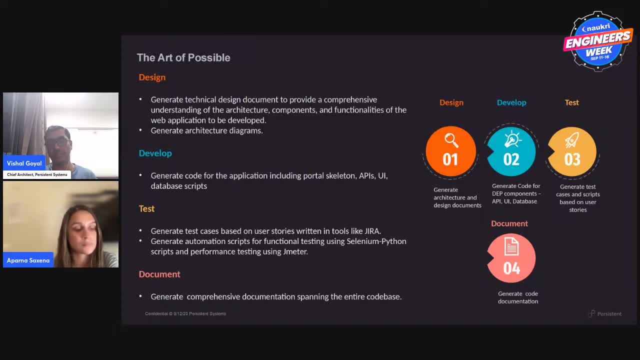 So typically this is your business analyst who will say: this is a user story. This is my design explanation. You will have a UI UX guy who will say: I'll use something like Figma to create wireframes and UI design. And then you will have a developer. 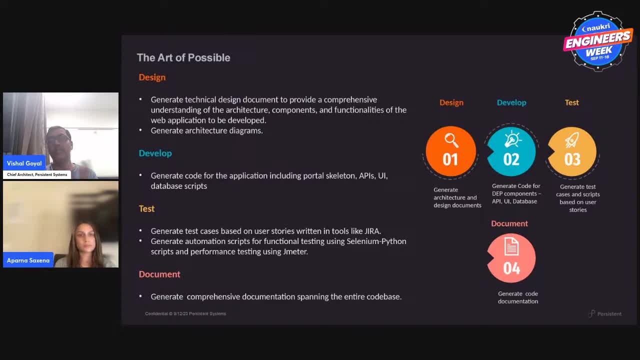 and then you will have a development team who will say: okay, based on this UI, I will decide a tech stack, I'll define an architecture, You will do a technical architecture diagram, You will do technical documentation and then you will have developers. 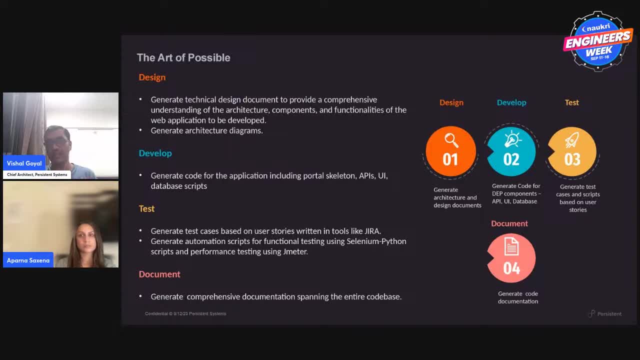 who will start writing the code, whether it is for UI, whether it is APIs and database scripts and so on, And then you will have a testing team who will either write manual test cases or they will write automation test cases using something like Selenium or maybe even other tools. 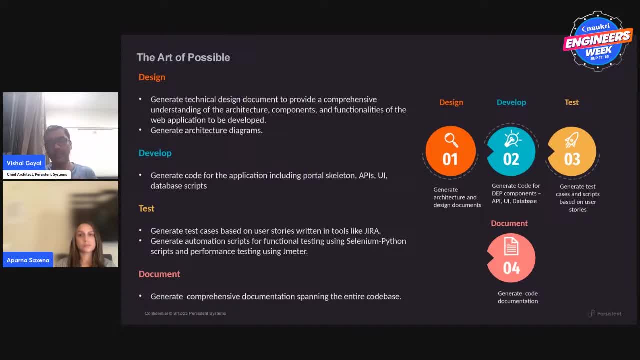 which are available in the market, And then you will also create documentation. Now, this is a piece which gets mostly neglected in a traditional SDLC, because one this needs a lot of effort. Second, this is something which nobody really gives a lot of importance to. 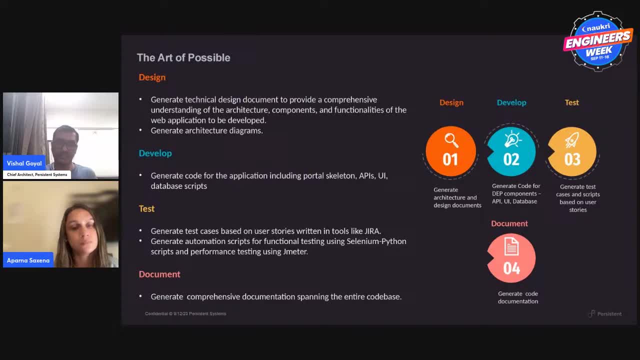 They'll say, fine, if documentation does not exist, I have the team who knows and who have the skills and will continue to maintain this. All of this is still being done today without GenAI, And all of this is getting really accelerated. 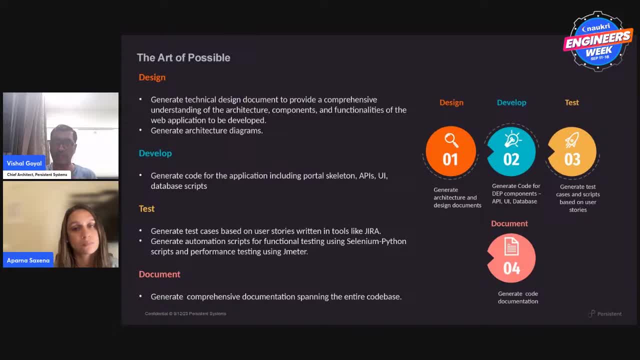 multi-fold- 10X, 15X, 20X time- with the help of GenAI- And that's what the art of possible which we want to focus on today- Can you generate architecture and design documents using GenAI? Can you generate documentation? 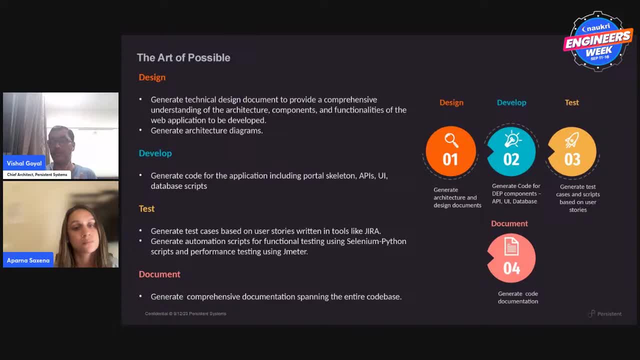 Can you write code for APIs and UIs and database? In fact, can you create a database schema? Can you create an entity relationship diagram? So I am not a database guy, I am just a UI guy. Can I still do some work? 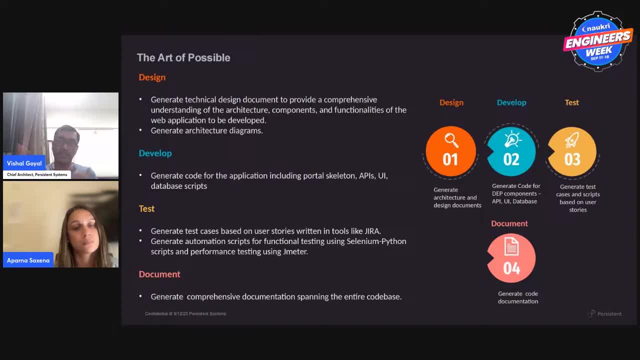 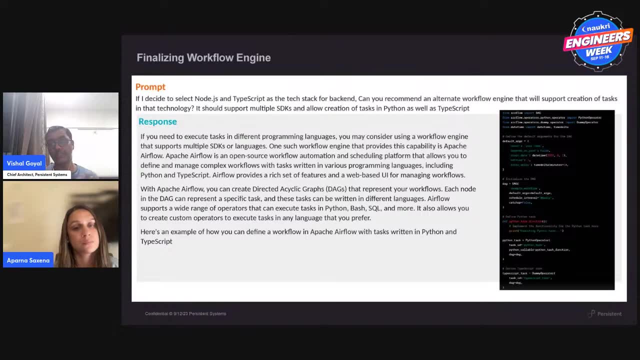 to create small database script- DDL scripts- and test my UI and things like that. right, That's what you will do in subsequent, So I'll give you examples, and some of these slides are pretty detailed in terms of prompt engineering, which is what we spoke about. 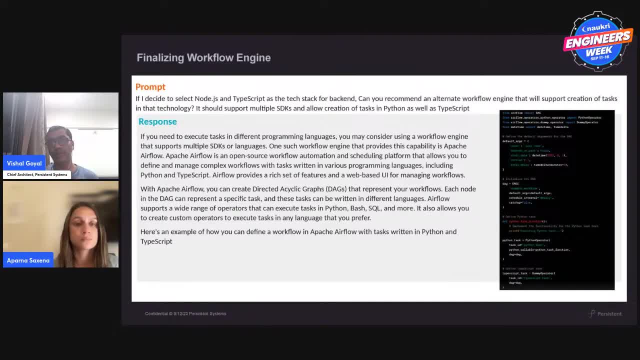 and the kind of response which you get. So this is an example where we are trying to build, let's say, an application And we are saying: I don't know if I use Nodejs TypeScript as a tech stack for a backend. 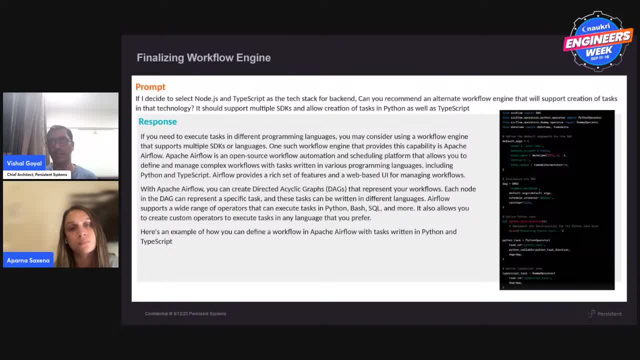 And I'm trying to have a conversation with GenAI to say: can you recommend a workflow engine? I don't want to use something which you have recommended, And this is a conversation which has already happened with some context, And I have picked up a conversation. 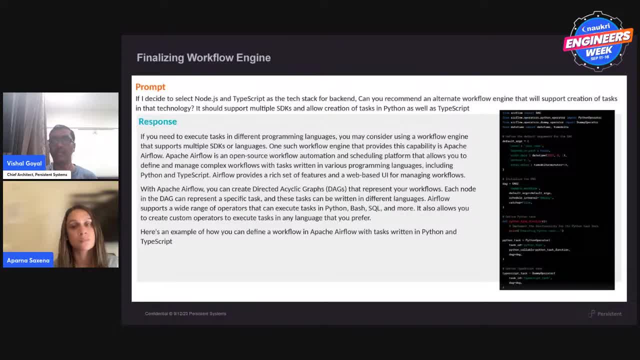 from between, saying I want to do something because I have decided to use Nodejs and TypeScript. Can you recommend something? And what this does, what GenAI does, what ChatGPT and BART does, is it gives you a good point of view? 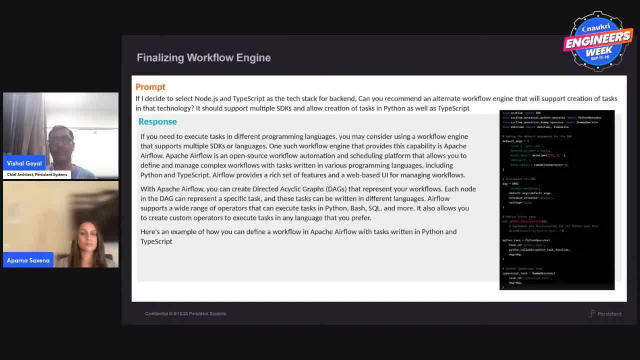 on what you should do. In this case it is saying Apache Airflow is what you should use because you are trying to do certain stuff. Since you want to execute tasks in different programming language, you should consider a workflow engine which can support multiple SDKs on languages. 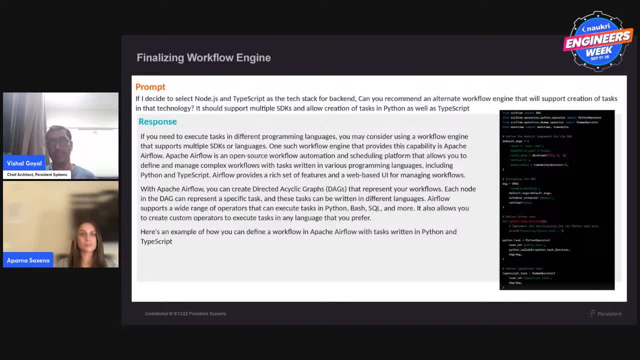 And version engine is Apache Airflow, And then it gives a little bit background And it also gives a code right here as a response that if you were to use Airflow, this is how the code looks like. So again, just take a pause. 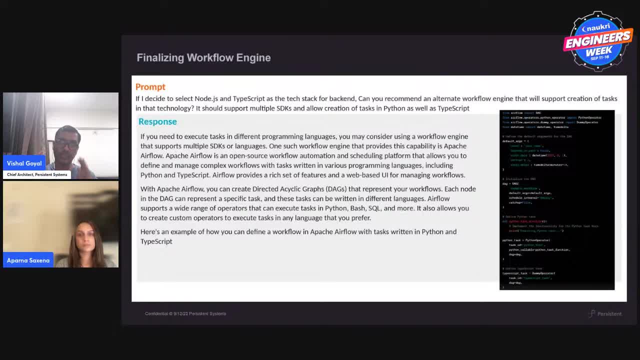 Look at. what I'm trying to tell you here is that it is not just writing a code, but it is also being able to get a very intelligent discussion. when you are trying to finalize an architecture, You're trying to understand which programming language to use. 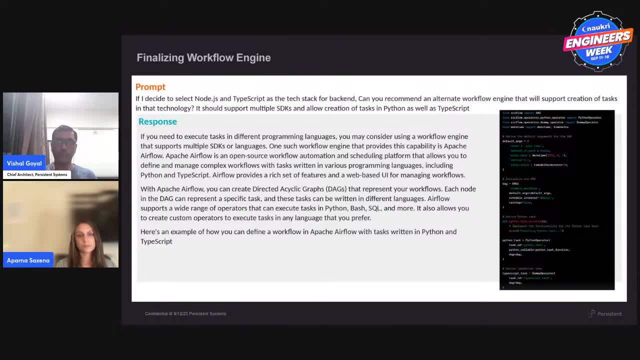 So between React and Angular, it is always a question mark. Should we use ReactJS, Should we use Angular? Which one is better? One is a library, one is in a framework, And someone who is expert on Angular will always have pros towards Angular. 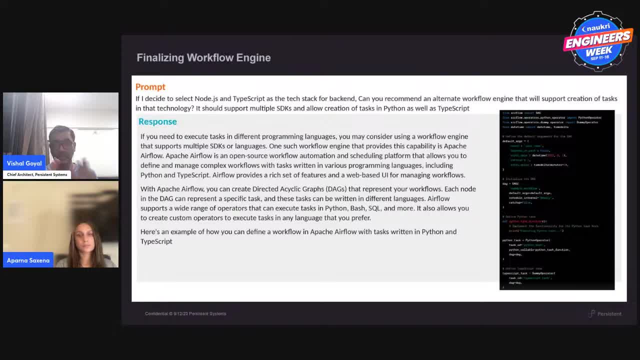 Someone who is an expert on React will always have a pro towards React. But as an independent person, based on your requirements, you can feed into a prompt, and that prompt could run into a couple of pages. if you want to, It could run into 10-15 lines. 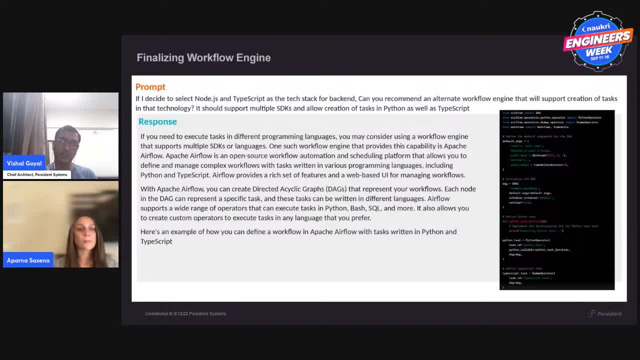 And then what you are able to do is have a very intelligent conversation with something like ChartGPT and BART, And none of this information is confidential. So none of this is user customer specific information. None of this is confidential. So, even if at this point in time, 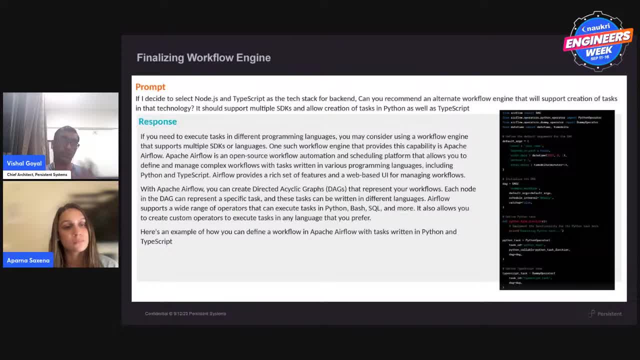 you were to use something like ChartGPT and BART, it is absolutely okay to do so, Because none of this, as I said, has any confidential proprietary information which you are feeding into this interface today, And this works brilliantly. We have done it ourselves. 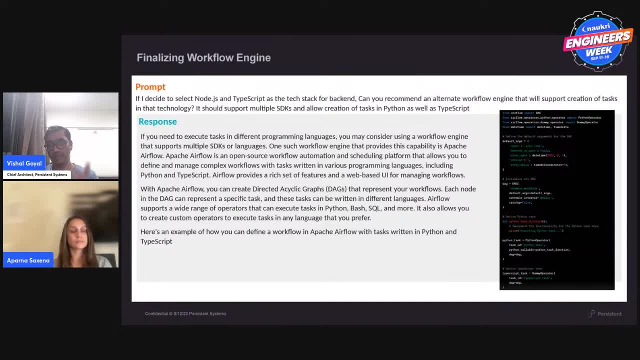 We have built our own application using this conversation, And what you see on the screen is a real conversation, which me and my team have done for building one of our applications. Again, I just spoke about this. So how do I choose between React and Angular? 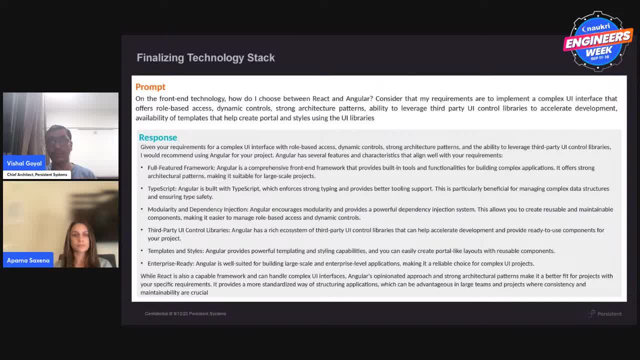 That my requirements are to implement a complex UI interface That offers role-based access, dynamic controls, strong architecture patterns, ability to leverage third-party UI control libraries and availability of templates to help create portals. This is the prompt, So the prompt needs to be intelligent. 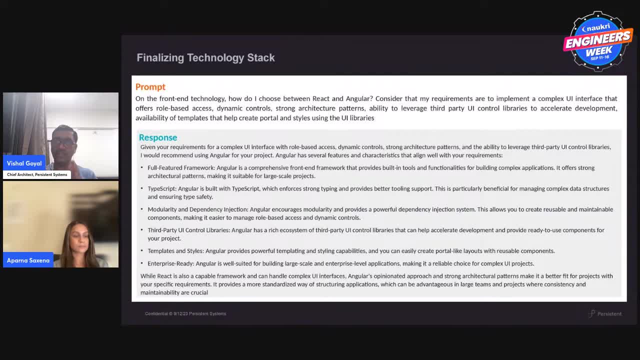 And that's why in my first section of the session I said prompt engineering is extremely important. So if someone doesn't know how to write that prompt which is there on the first top section of the screen, then obviously you are not going to get. 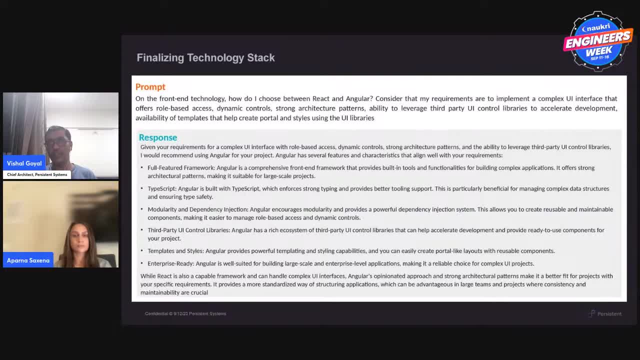 this intelligent response bar, So to be able to use GenAI, to be able to use ChatGPT, to be able to use BARD or any such solution, knowing what to write, how to frame it, while this is plain English, 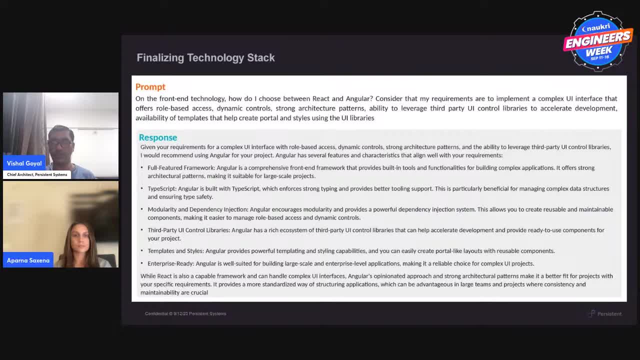 but then from our experience over the last six months talking to different technical people, technical people struggle to write plain English. They know how to write a code, They know how to debug a code, But when it comes to writing plain English language, then this is a little bit of creativity's work here. 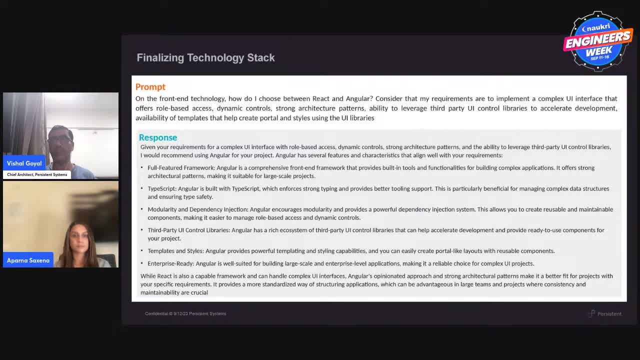 And this is something which is not every technical developer is comfortable with writing, But with GenAI, this is something which needs to be built as a skill And what you see based on. So, first, it basically comprehends and understands what we said and it is basically affirming it again. 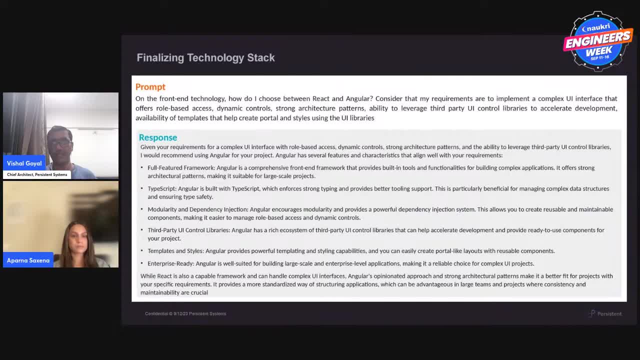 So you said you want to build a complex UI interface, and this is what you should do. Angular has several features and characteristics And it is recommended you should use Angular. And why you should use Angular is what it has listed down, And it is also doing a little comparison to say. 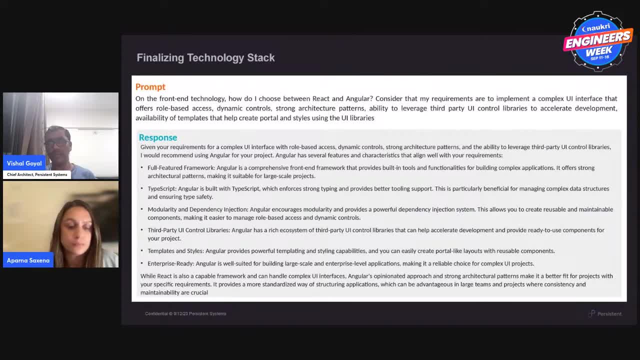 while React is also a capable framework, Angular is far better And in our case, we had already built this platform before GenAI and we had chosen Angular, And this has just re-emphasized and reconfirmed our architect's belief system that Angular is better than React in our case. 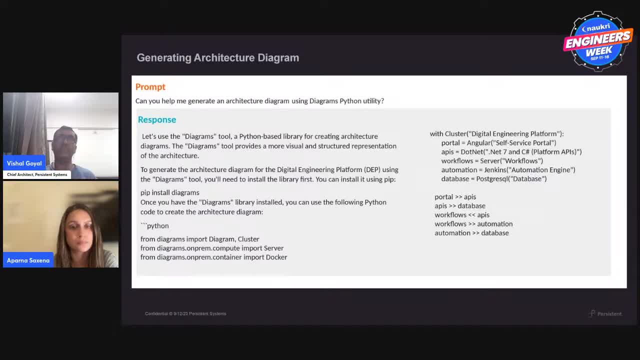 Again. now we are trying to do an architecture. So remember when I said ChatGPT 3.5, the open source one. you cannot really generate a diagram. It can only work with text-to-text, But what you also have is utilized diagrams. 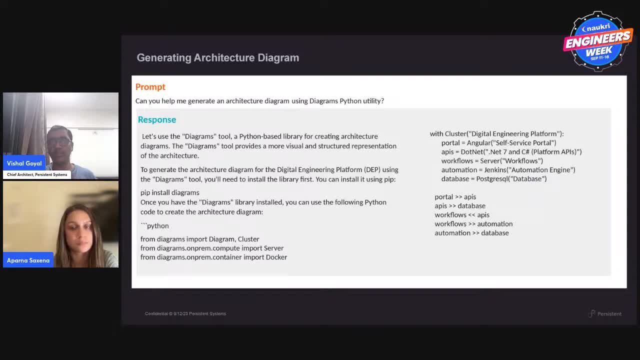 and tools available which you can use to integrate with ChatGPT to be able to generate a diagram, And that's what this promises While I'm saying: help me generate an architecture diagram using diagrams Python utility. That's all I have said. 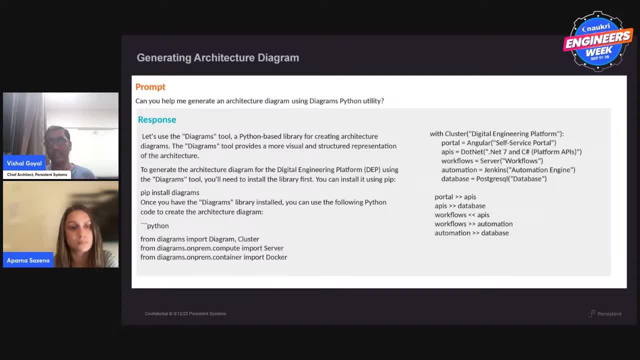 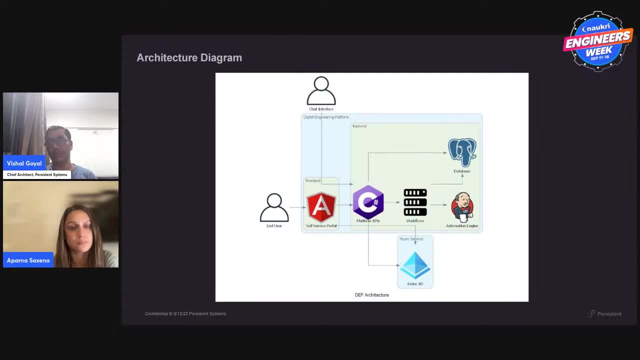 And then what it does is: it understands what diagram tool can do, It generates a code- and this code is based on the earlier conversation, which I would have done- And then what I get as an output is this diagram. So this diagram itself is generated by ChatGPT. 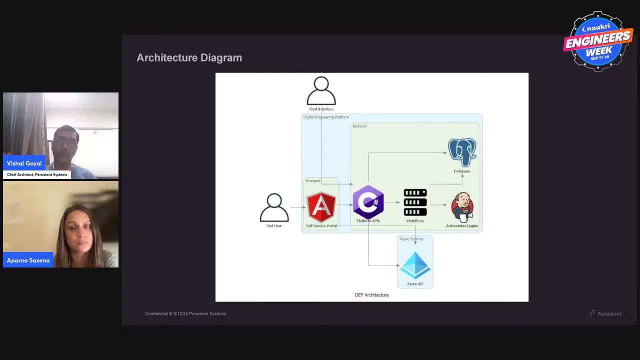 It is not generated by ChatGPT 4.0 or any other tool. This is generated using the free version of ChatGPT, which is 3.5. So certainly possible. to do that You need to know the art of prompt engineering. 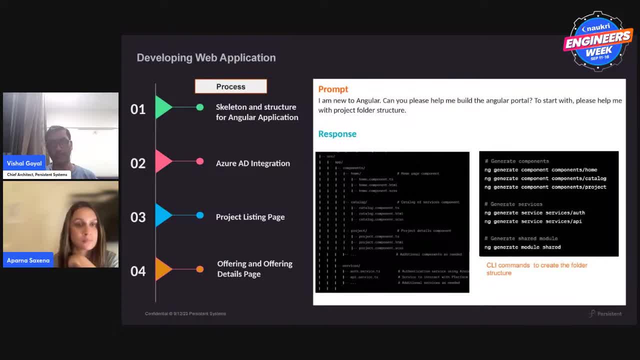 I'll go a little fast and then, so that we can have more time to take up questions. Now, how do you develop a web application? So what we have done is we have been able to generate a code for an Angular application, What you see on the screen right now. 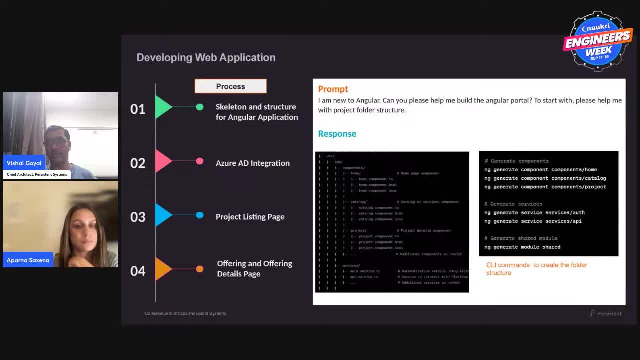 is the complete directory structure and an architecture of CLI commands. I can run the CLI commands in my Visual Studio code and create the entire architecture. We have generated code to do an Azure AD integration and we have created multiple pages within my application to be right from ChatGPT. 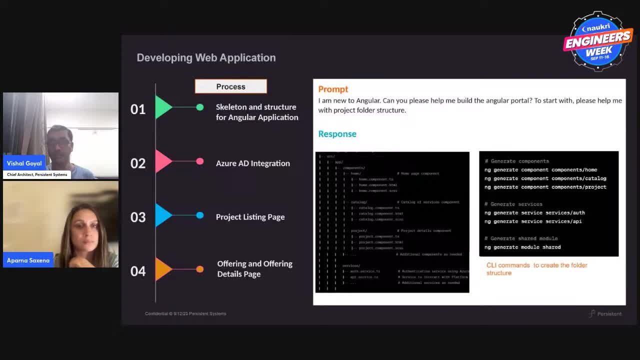 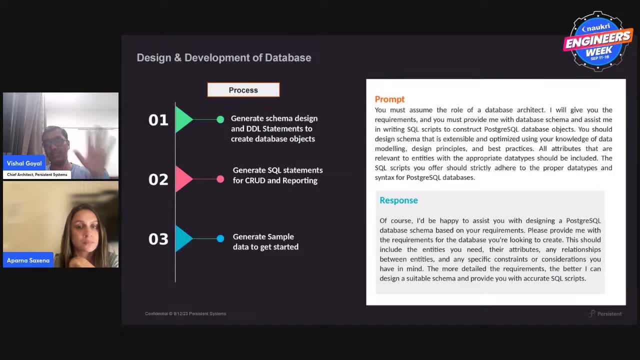 without writing a single line of code. Is that possible? Of course this is possible today. Again, database. So I'm covering the aspects of it. What was the design? Then you had the development and now I'm trying to create a schema design. 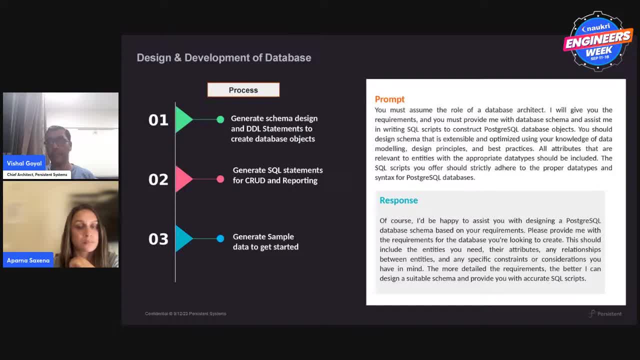 So again, you see the prompt. here. I've given a couple of important things. I want to use a PostgreSQL, I want you to create SQL scripts and I am a database architect and I want you to do all this. And it says I would do this for you. 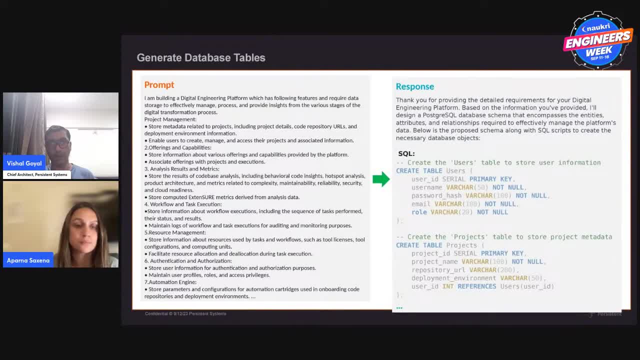 and it generates the scripts. Now I have given a long prompt. You see the size of this prompt. here I've defined what I want you to do and it basically generates my script for creating tables with primary keys, foreign key, and all All this is again done using ChatGPT. 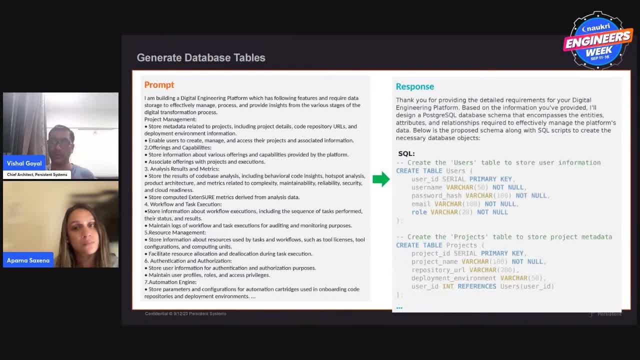 So people who are there on the call, who have not done a lot of this work and who are getting surprised, please don't be surprised. That's the art of possible. That's the aim of this session, That was the messaging. So this all is possible. 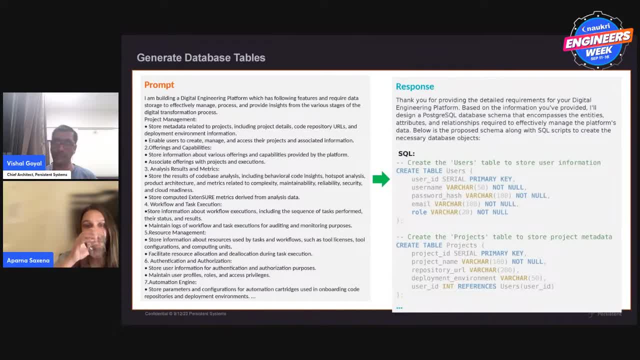 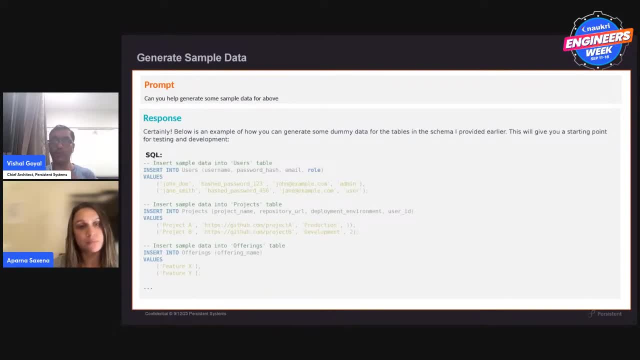 and this is what is real. We have done it. I have not copy pasted these images from Google and telling you this in the session. Again, you can create sample data, So a lot of times you will say, okay, now I want to populate the data in my tables. 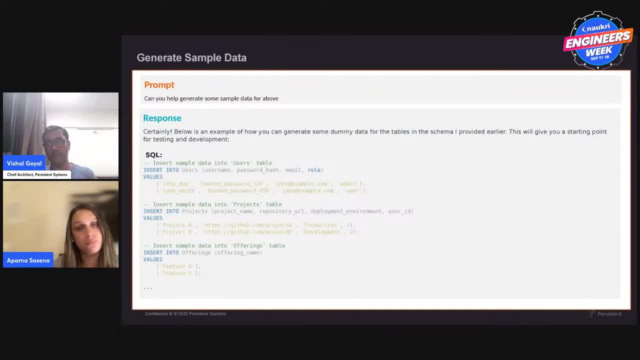 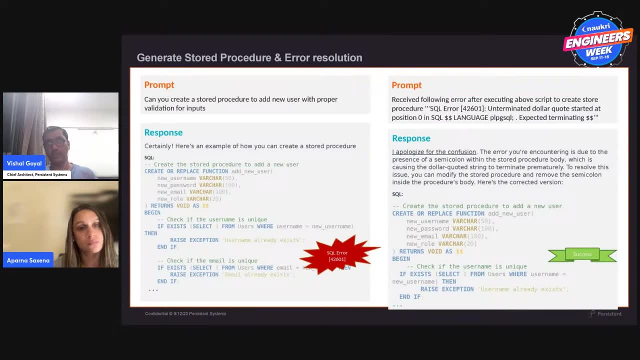 which I have created earlier. So it has created your insert scripts. now, using the same tables, You can create stored procedures and you can also resolve problems on those procedures. So if you have generated a procedure and you say I tried executing this procedure and I got an error message, 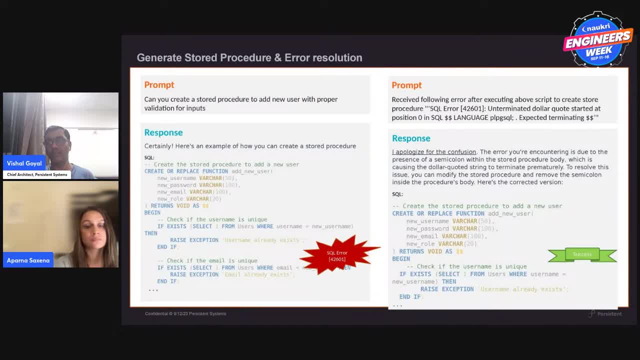 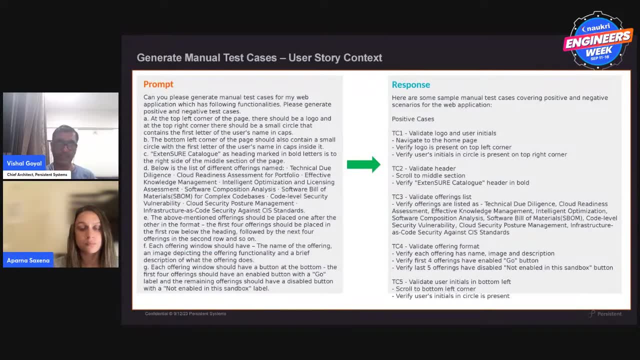 it will then fix that code and it will give you a modified procedure code which will fix that problem. So then again, it's a conversation which you are doing. How do I generate manual test cases? Again, you give a prompt right here and now. you could give this prompt in Jira. 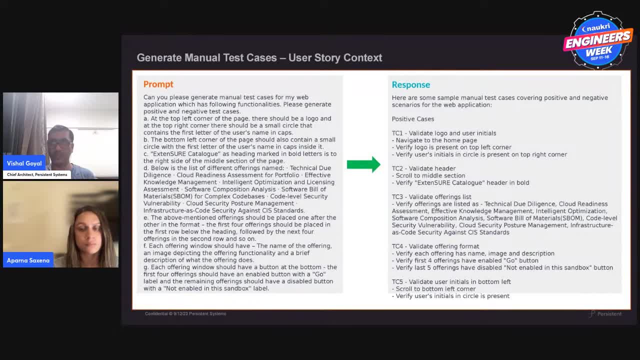 There are plugins available with Jira. So Katalon has a plugin available in Jira which can help you write this user story in Jira and then it will create these manual test cases and then your tester can start. So imagine you have testers who have never done testing. 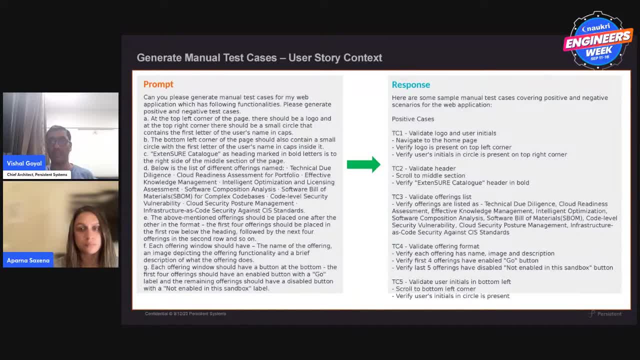 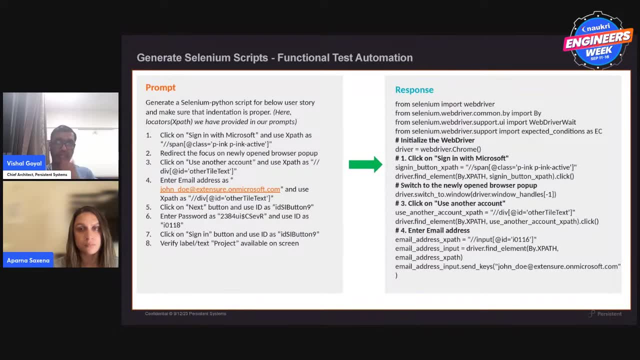 and you are a seasoned tester. You give this to someone and they would be able to start doing testing very easily for any application. This is generating a Selenium script, again for Python, So I gave some context to say I want you to do this. 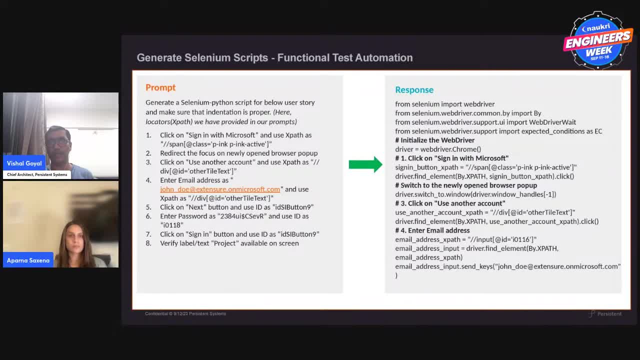 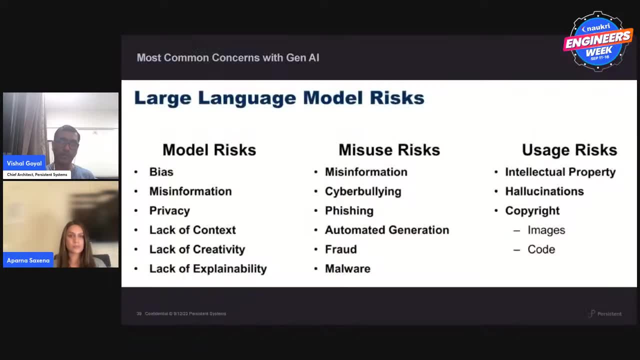 I want you to use a dummy email ID and password and it is able to generate a Selenium script for us. Last section: where do you start? What do you do? Some of the things very important for people to know that, while GenAI looks brilliant, 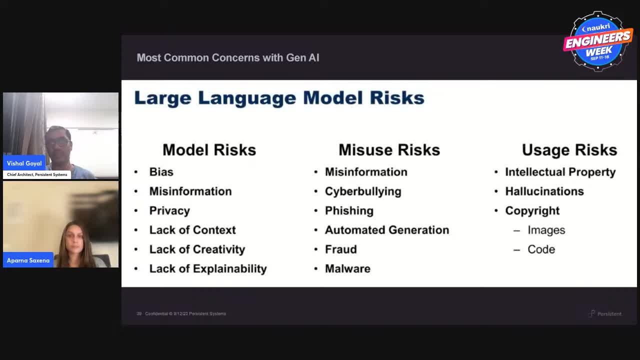 and it looks fascinating. there are things which are important to know. It has bias So it can hallucinate. So a lot of times you will ask it a question and it will generate a response which will look extremely real. You will say: can you give me a company which does this? 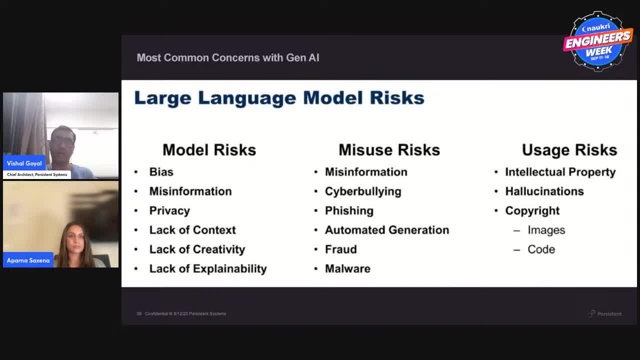 and it will make up a company to say company. Vishal Goyal Incorporation can help you do this. This is based in Pune and this is a million dollar company. All that is hallucination and it is not real. So very important for you to know. 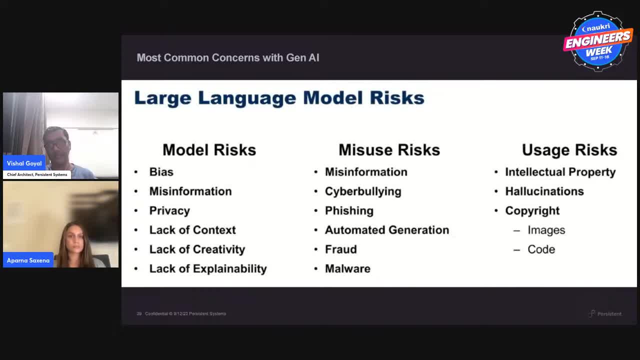 what content gets generated and validated. It can obviously do bullying, So it can start creating fraudulent activities and it can create malware and a lot of this stuff. So this is important for people to know: that while you are using it, it can generate a code which has copyright issues. 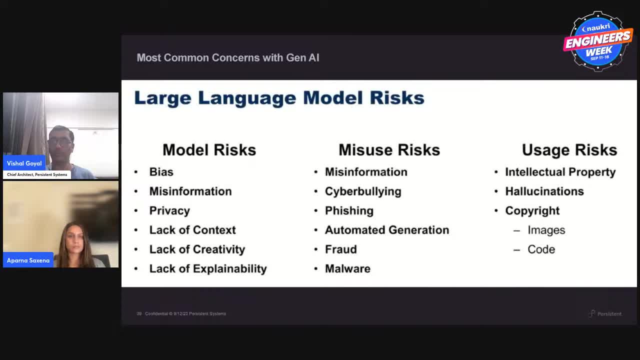 and you have a lot of litigations which are already filed by people from the open source community on open AI and others- that you use that code which was there in open AI, open source, and you use that to train your model. and this is, this is. 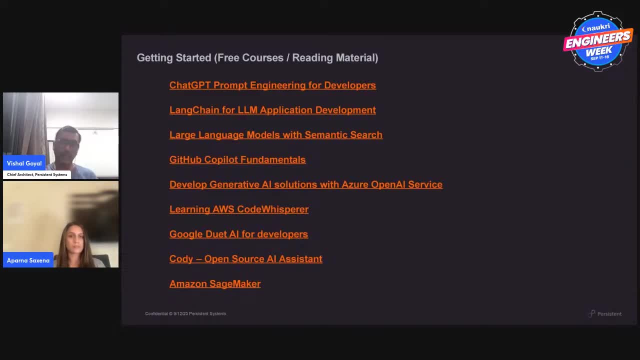 copyright violation of our open source code. Now, these are some references and I may be some of these will get published later on after this session, But what you should look at is there are courses available on deeplearningai, which is managed by Andrew Ng. 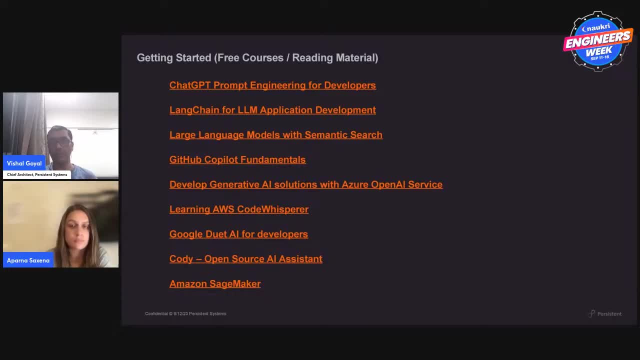 and these courses are available free of cost for you to be able to do. and ChatGPT, Prompt Engineering, is your first course, which people should do it, and so on. It is a very small course, short course, which you should do, but there are other others as well. 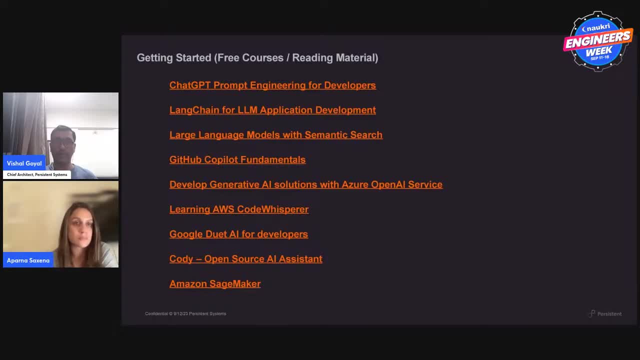 GitHub Copilot- Again- people who want to start doing coding and development using from ID- Very important to you. Again, this is a free course on microsoftlearn, So go to microsoftlearn and start doing this course for Copilot. Azure Open AI Service. 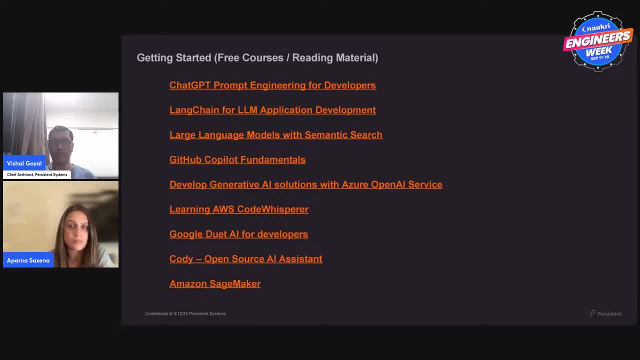 Again a course available on microsoftcom which will tell you what open AI service is, how you can consume this into your Python code and things like that. Like you have Copilot from Microsoft, you have CodeWhisperer from AWS, So there is a course available on AWS website. 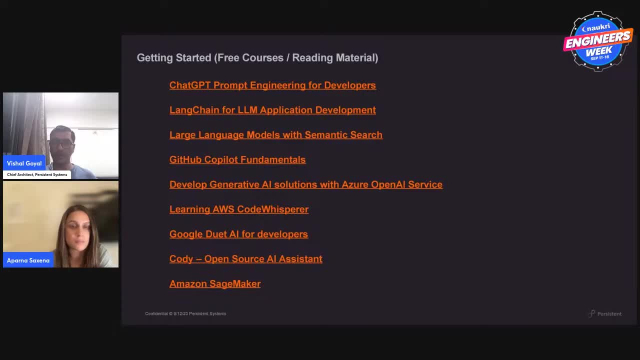 And you can go there and start doing that. They also have a curated hands-on session available. You can do that online and they'll give you a playing ground where you can play around with it. Similarly, Google has something called Do It AI for developers. 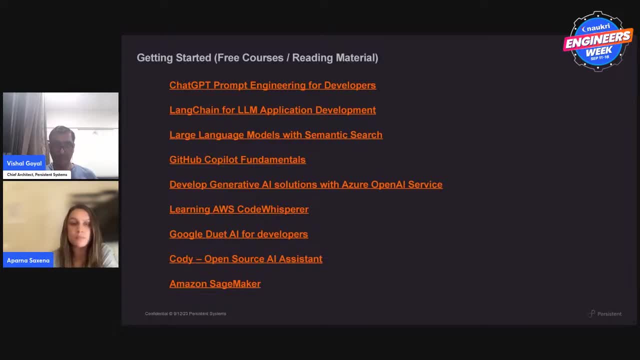 You can sign up for the beta and try it out. Kodi is from Sourcegraph, So there is a company called Sourcegraph which has released Kodi. This is open source, So you can go to sourcegraphcom. sign up with your public githubcom account. 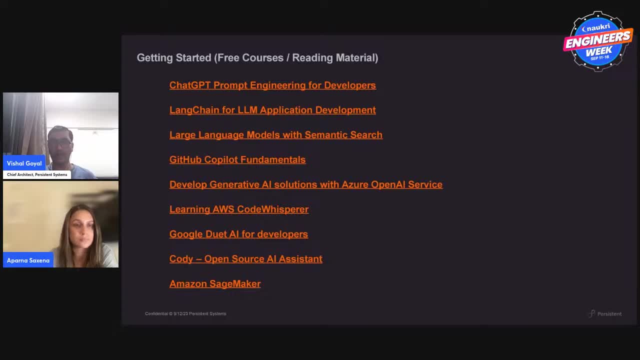 and use Kodi on any public report, So it will help you, And it is probably the only browser-based AI system available today. While Copilot Do It and CodeWhisperer all work in IDE, this works in a browser itself. 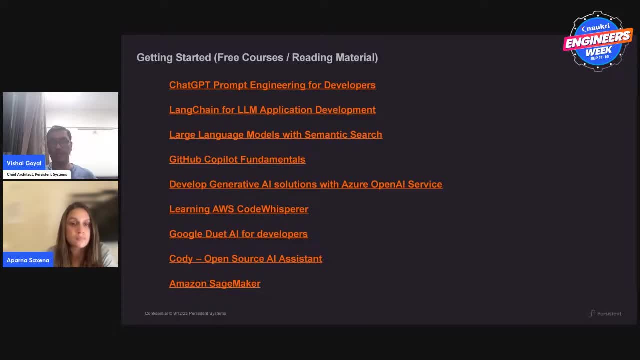 And then SageMaker- again important platform as a service offering from AWS which people should do if they want to get a little deeper. That's what I wanted to do today. I hope people found it informative. Oparna over to you. 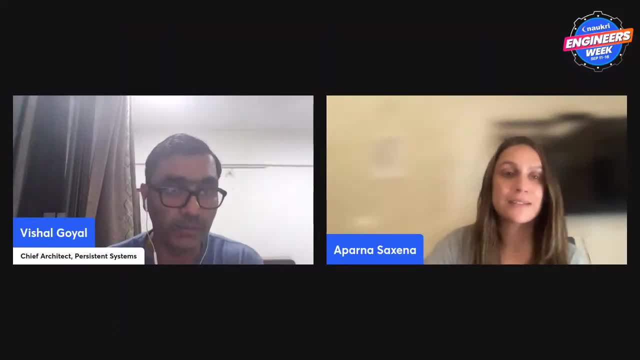 And we can take some questions from people Absolutely. Thank you so much, Vishal. That was deeply informative And I'm sure there are many attendees who are going to take a lot from today's session. There's a question that I wanted to bring up. 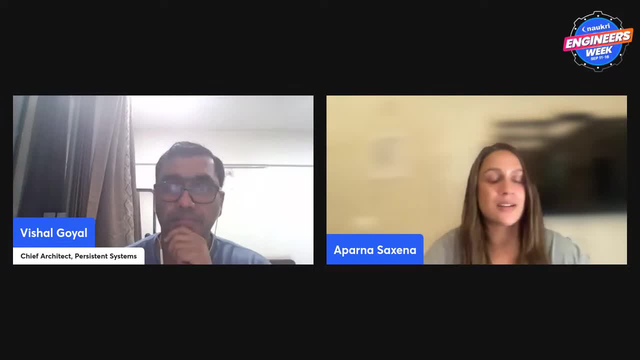 specifically in the skill building segment. So how should engineers think about building skills in AI and where would be the right place to begin? Yeah, as I said, so go to deeplearningai. today. There are courses available on what is prompt engineering. 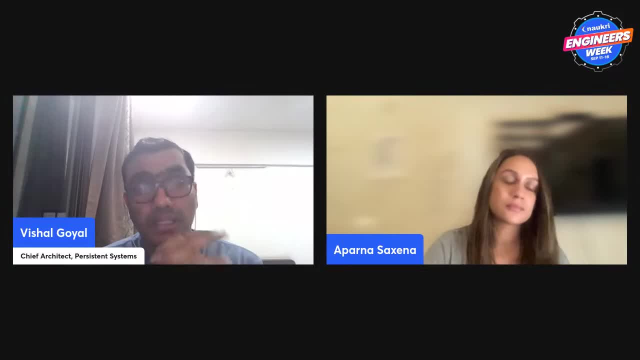 using ChatGPT. what is LanChain? So, if you know Python, if you're a Python developer, something like LanChain would be very appealing for you, And that's how you should start right And the most simplest is go to ChatGPT. 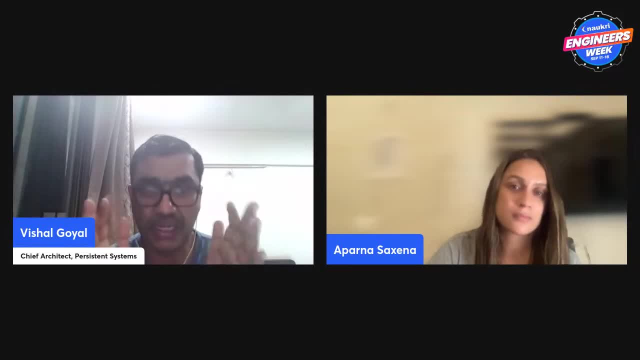 create your account using your Gmail ID or whatever ID, and start talking to ChatGPT. You can do it on a phone while traveling from office to home, home to office. You can do it sitting on a laptop. It doesn't cost you anything. 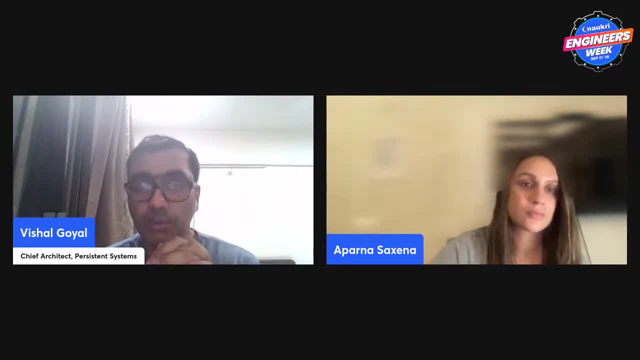 It is completely free And that's how you will learn more and more as you start doing it, And there are recipes available for doing prompt engineering. What are the right prompts If you go to promptengineeringai? there are a lot of recipes available. 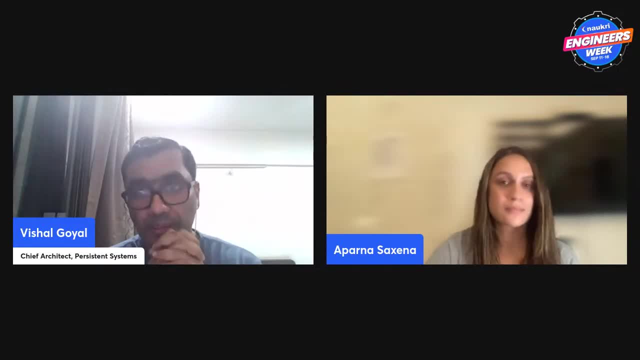 So, Panna, to me that's the best way of learning how to use GenIAI. Absolutely, That's a great tip. Another thing that I wanted to ask is that engineers often seek real world examples to comprehend the impact of emerging technologies. 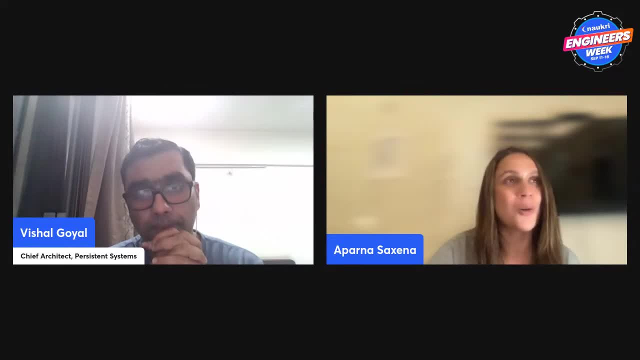 So if you could share a specific real world example of how generated AI has improved a software development process or elevated a software quality, that'd be really helpful. Yeah, So if you see, when software engineers join an organization like Persistent, they go through a training. 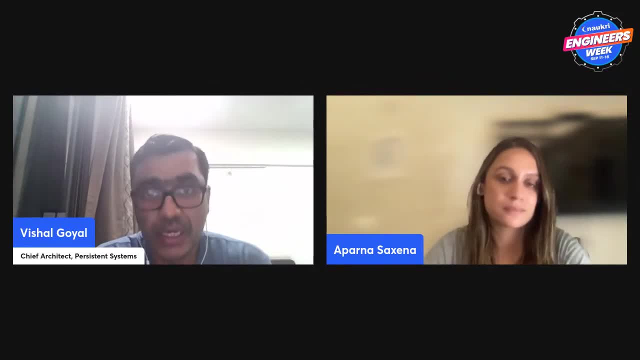 which is basically a foundation training on different programming languages, And it takes some time for organizations to deploy them on projects just because of the skills they need to develop and the amount of knowledge they need on a particular programming language. With GenIAI, what we are seeing right now- 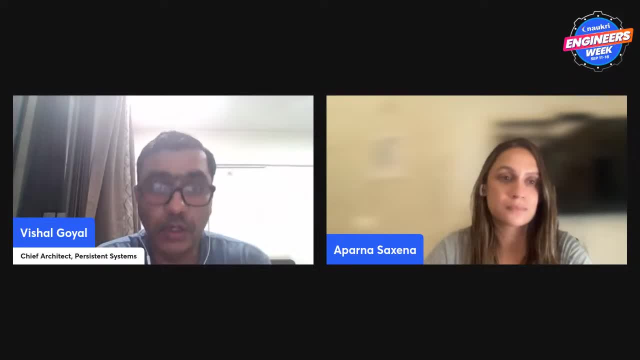 is that the ability to be able to deploy these engineers who have joined us into projects is much faster, Because they would be able to generate code or write code, explain a code which already is there much, much easily. That's one example. Second example which we are seeing is: 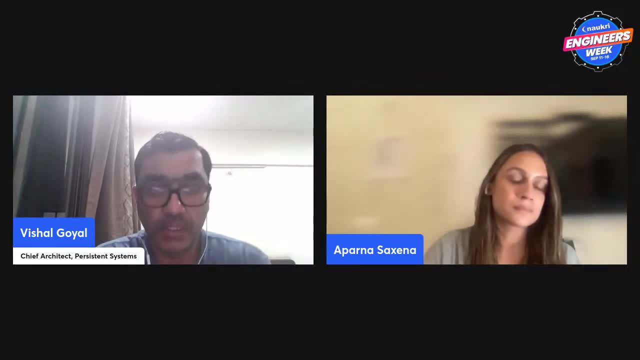 at Persistent. So let's say we are working with a customer who has another vendor working on our application And for some reason customer is not happy with that vendor and they want to transfer that application and do work with Persistent And Persistent is going to take over that product. 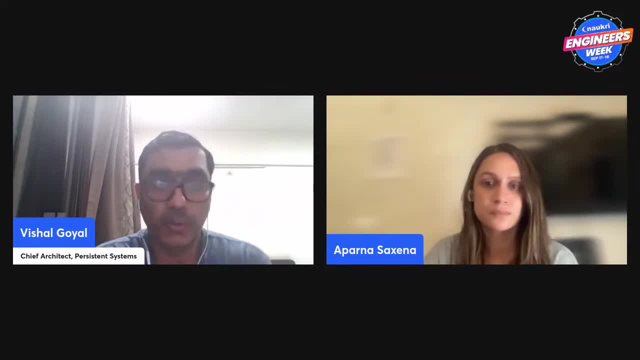 which runs into a million lines of code. And imagine there is no documentation available for that particular application And it's a hostile takeover. The existing vendor is not ready to do any knowledge transition. So how do you understand that code for developers? And that's where GenIAI is able to explain. 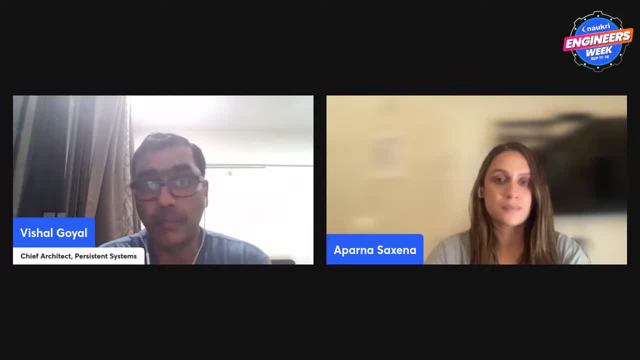 that code in function by function, lines by lines, and be able to really improve the developer productivity in understanding that code and refactor it and modernize it. Another third use case is: so in my experience, what we have seen is while developers write code, 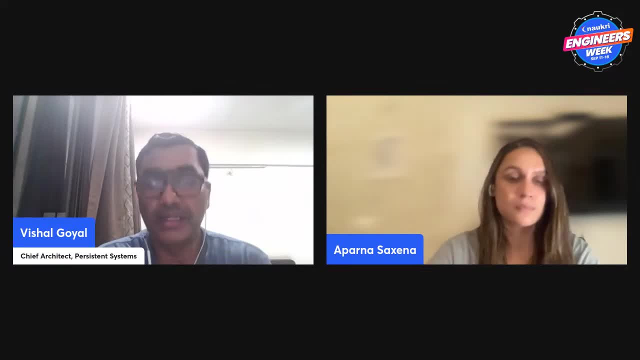 they do a fantastic job. They don't write unit test cases And that gets ignored most of the time. But if that needs to be improved, now with GenIAI you can actually generate unit test cases, improve the code quality and improve the code coverage. 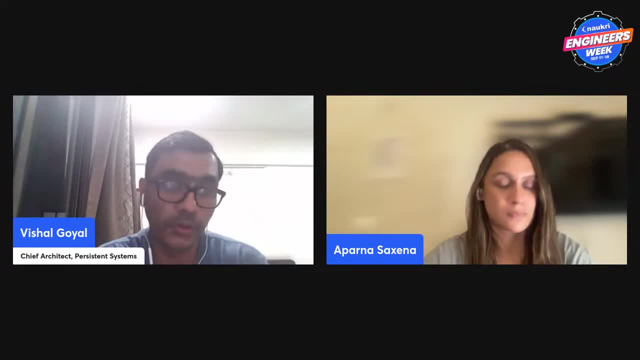 of unit testing before. So those are three good use cases which are seen in the context of software engineering very prominently coming to us over now. That's great, And what would you say is specifically for the audience that are engineers seeking job opportunities, if they're looking for an understanding. 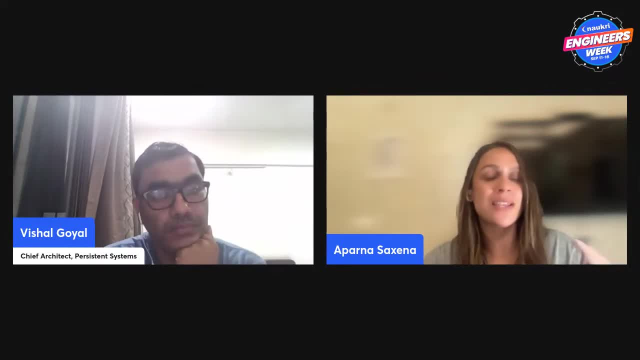 specifically with Persistent. how is AI being currently leveraged at projects at Persistent at this point in time? We did go through it, but if there's opportunities that are upcoming, we'd love to hear about those. Yeah, So Persistent is heavily invested into GenIAI. 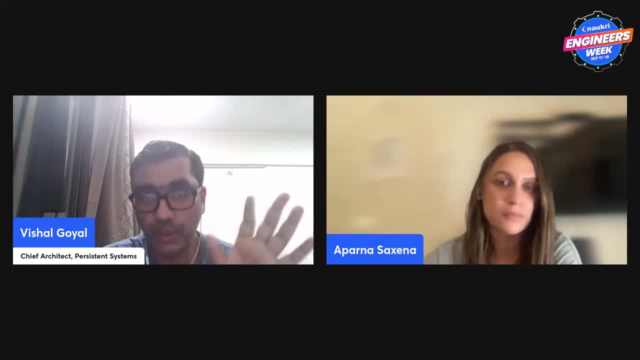 So we have a dedicated CTO group which does a lot of work around the LLM. I am part of a team which does a lot of work around application development and application engineering around GenIAI- So very heavily focused. We have excellent partnerships. 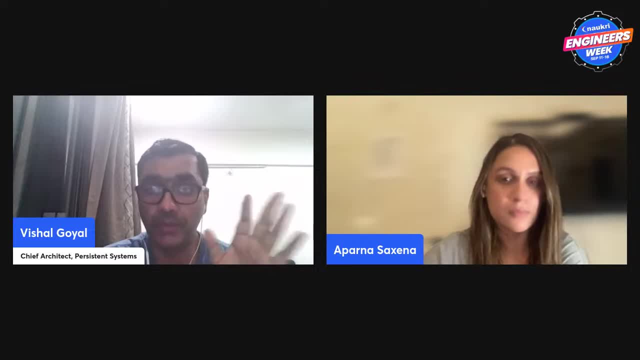 with all the hyperscalers. So if you look at Microsoft, we have dedicated partnership to use Azure OpenAI. If you look at AWS, we have early access to Bedrock and SageMaker Jumpstart. If you look at GCP, again, we have a dedicated partnership. 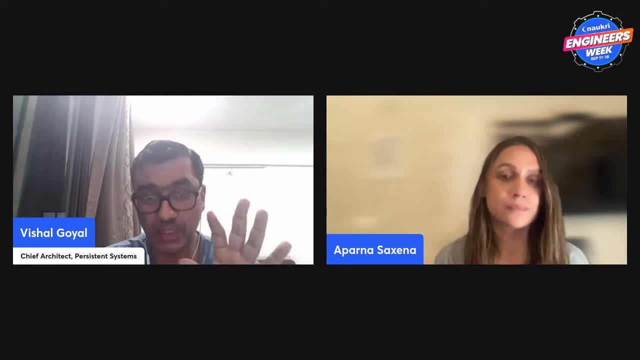 with the Google Cloud platform. So these are the areas where we have been primarily heavily invested in. And then we have a lot of other partners where they have started adopting GenIAI into their products and we are then using their products to give this advantage back to the customer. 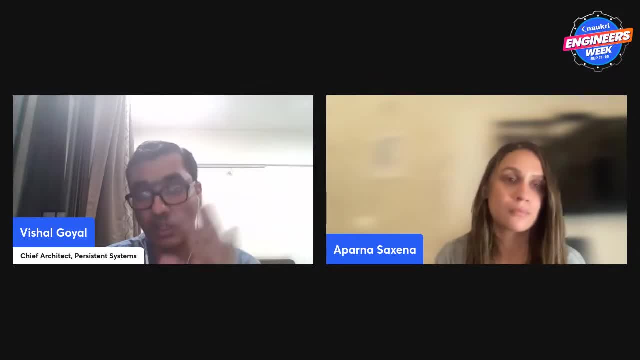 But if people on the call who are looking at joining Persistent, who are looking at getting into GenIAI, as I said in my slide deck, I would request you to start building some of these skills: prompt engineering, retrieval, augmentation, generation, tokenization. 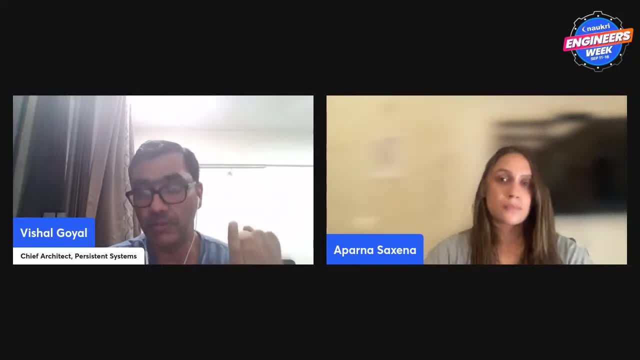 encoding, decoding, knowing how CodeWhisperer works, knowing how Copilot works and knowing how ChatGPT works. So today, when we talk to a lot of engineers, they just don't know even how to do a prompt engineering with ChatGPT. 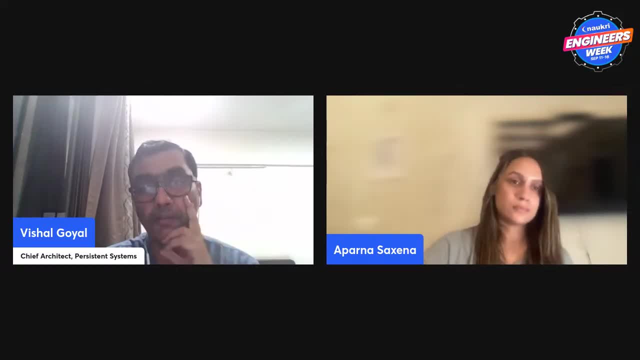 I guess those are basic hygiene skills which we expect people to know now, Absolutely. We do have a question from one of the attendees who's asked: what is the process to use GenIAI for Azure, Google AWS DevOps? If you could elaborate? 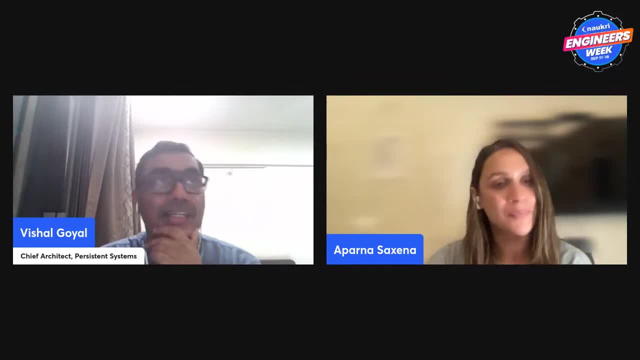 on the process of that. that'd be really helpful. Yeah, so very simple. If you wanted to use CodeWhisperer today, it is completely free- Go to AWS CodeWhisperer. So open Visual Studio Code or IntelliJ, whichever ID you use. 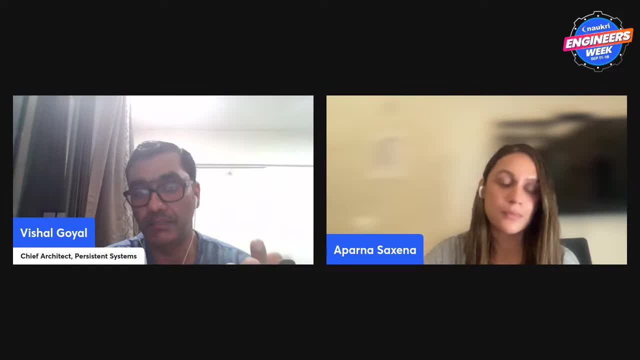 Install the extension. It is called AWS Toolkit. Create a builder ID using your Gmail ID or whatever personal ID and start using it. All the capabilities generating a code, adding a context to a code. You can download a public resource repo from GitHub. 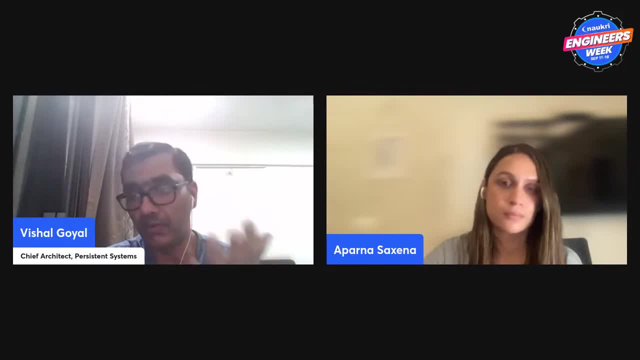 So let's say, you don't know how to write a code, download a public repo from githubcom into your ID, clone it and start using it. So that's AWS right And DevOps so DevOps. things will remain the way they are right. 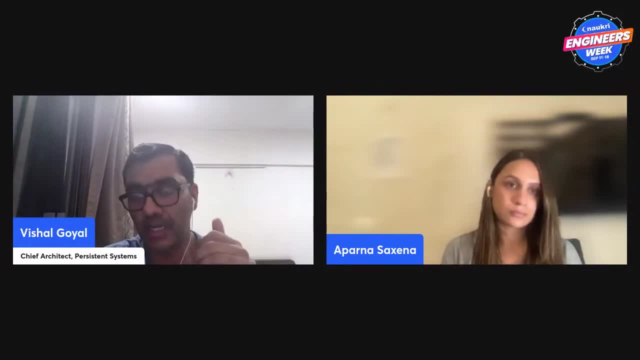 So DevOps is not changing with GenIAI. If you want to use Azure again, you can go to Azure. create a free account, use an OpenAI. So even OpenAI gives a free account for some tokens Beyond a certain token. 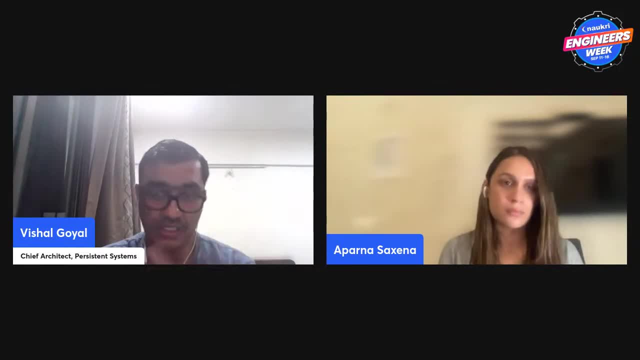 obviously there is a limit, but you can use Azure OpenAI. GCP again offers free credits for being able to use. So what you need to know is there are free services available for each of these hyperscalers. All you need to do. 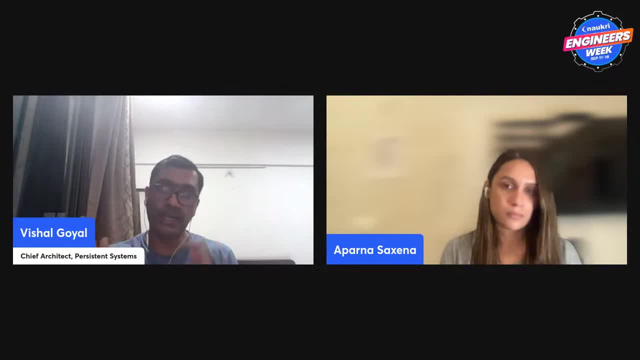 is be able to use them to a certain extent. Beyond that, depending on how much you want to really invest in your career, to build it, you can sign up. It's a nominal amount for using this, even on a commercial site, Like a lot of us have created. 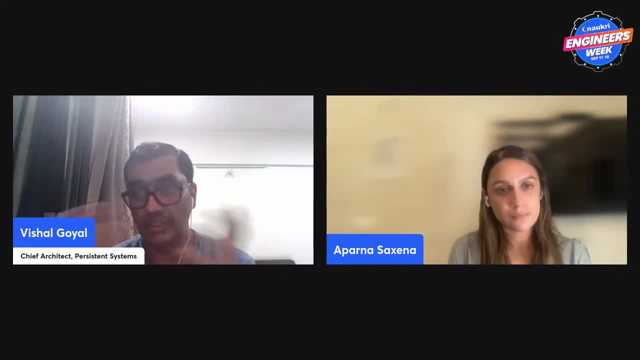 a commercial account with GPT-4, which is $20 per month, And we use that extensively for doing whatever we want to do For people who are really serious and they want to invest some money. they can certainly do that as well. 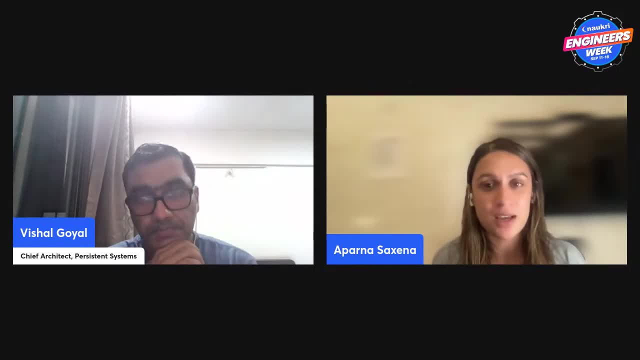 Fantastic. Another question from the audience is around business analysis. So for business analysts, how could they leverage ChatGPT in their work if you had any tips for them? Yeah, So, depending on what is that you do as a business analyst in software engineering? 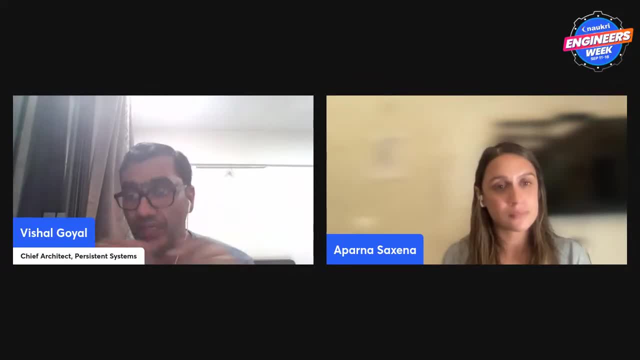 what you would want to do is the work which I showed you in the design phase, right? So if you have a requirement in mind, you went to a customer and customer gave you a requirement and you wanted to get a little bit understanding on what that really means. 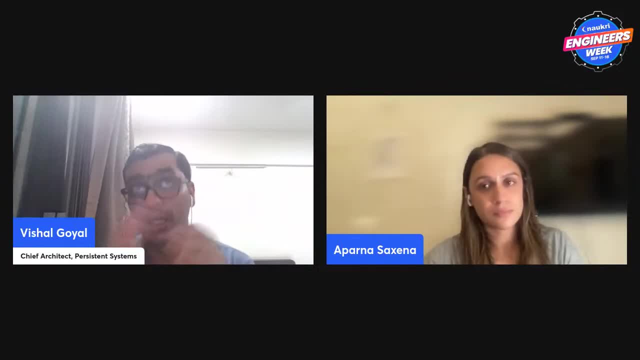 you can do that prompt discussion with ChatGPT. You wanted to give a little bit more deeper requirement to your development team or to your designing team, the UI UX team. you can certainly refine your entire design or your entire requirement based on something like a ChatGPT discussion. 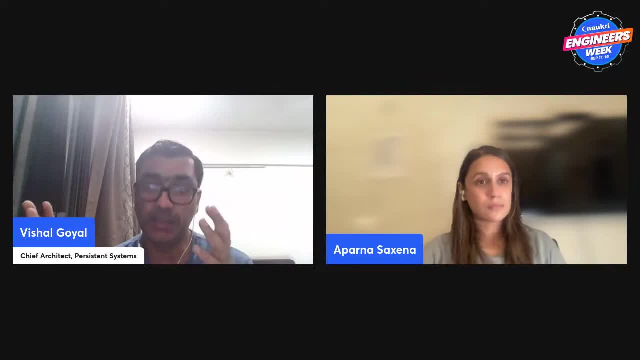 So what? what GenAI and the likes of ChatGPT and BARD are doing for business analysts is it is helping you define your requirement for two sentences, three sentences, to actually a entire page of requirements. right, That's what business analysts should be able to do. 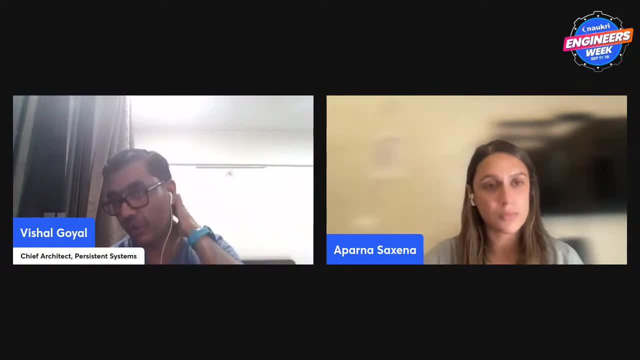 If you want to create content for going to a meeting- so you're a business analyst and you are meeting a customer and you wanted to get a little bit content created for your meeting- you can certainly do that as well with ChatGPT, So possibilities are endless. 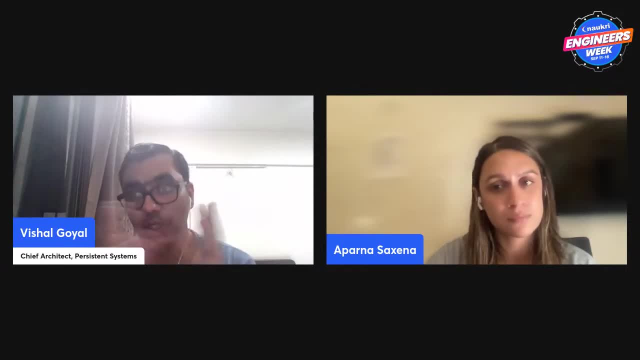 As we said, the art of possible is there. You just need to know how to converse in your area. And the more you use ChatGPT, the more intelligent you will get, because, based on the responses, you will know what it can do. 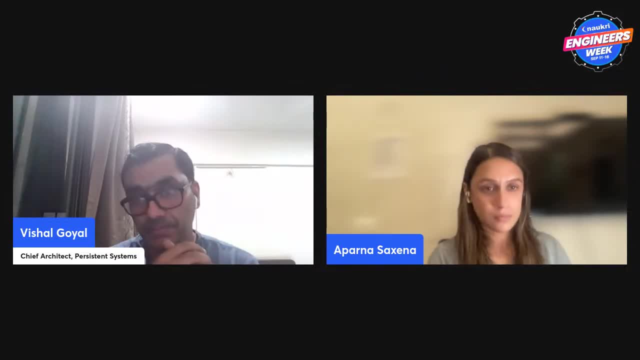 what it cannot do and how do I ask for the questions? Fantastic, Before we wrap up this session, I think I can do one final question, and that would be around: how do you see the career in AI evolving over the years In the next decade? 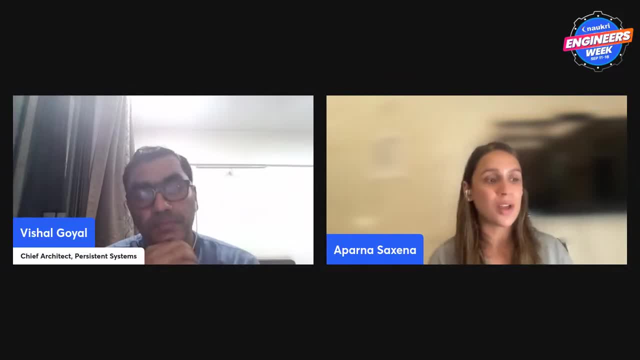 I think a lot of the engineers attending this session would like to know how quickly they need to upgrade themselves and what kind of upskilling is going to be required once they choose this path. Yeah, so Swabhana AI is here to stay. 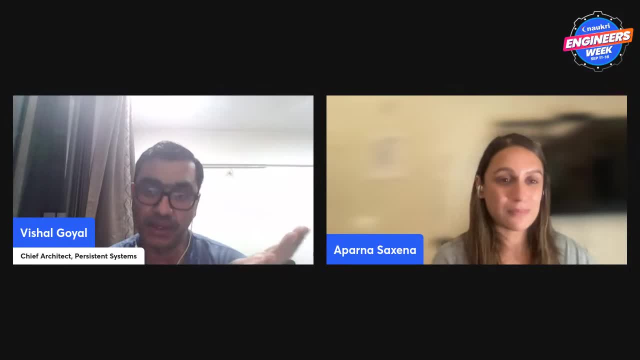 So people who don't look at GenAI, they are definitely missing out on something which is an integral part of software engineering today. Any organization you join today- whether you join a startup, whether you join an enterprise like Persistent, GenAI will continue. 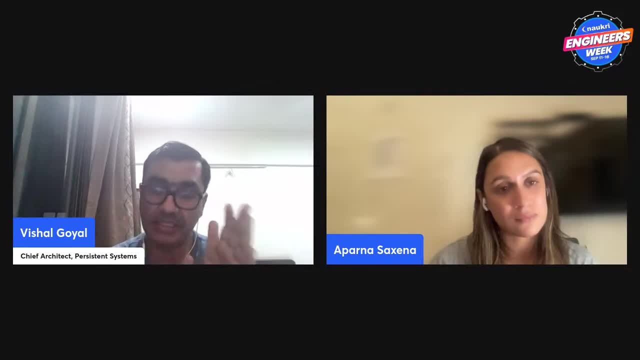 to become an important area, no matter whether you join us as a tester, whether you join as a developer, whether you join us as a business analyst or whether you just join, even in teams like legal and corporate teams, and even as part of the finance teams. 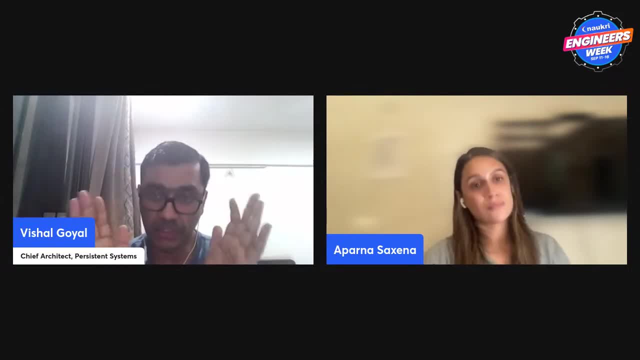 GenAI will become extremely important right. So that is the first important aspect for you to know. This is not something which is nice to have stuff. This is hygiene, now as part of your professional career. Now, what do you need to know? 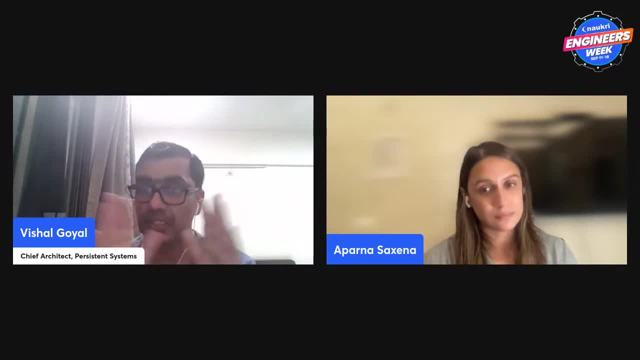 As I said as part of my deck, as a part of my session, there are important. So if you are a data scientist and you already are hardcore into machine learning, you should look at doing the fine-tuning aspect of it. You should start getting into. 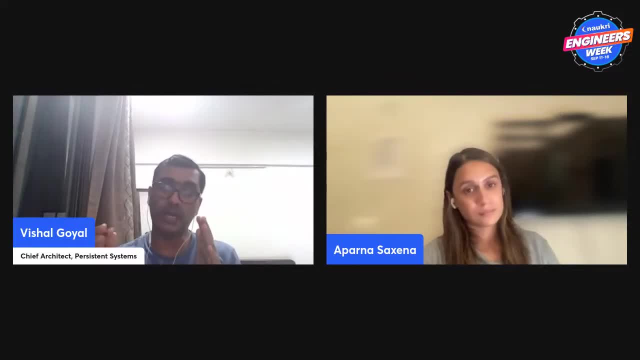 something like AWS SageMaker, the Jumpstart and the AWS Bedrock stuff, right? So that's for people who are already AI experts, who know machine learning, who know deep learning, who have been doing Python programming and do know the algorithm using XG Forest. 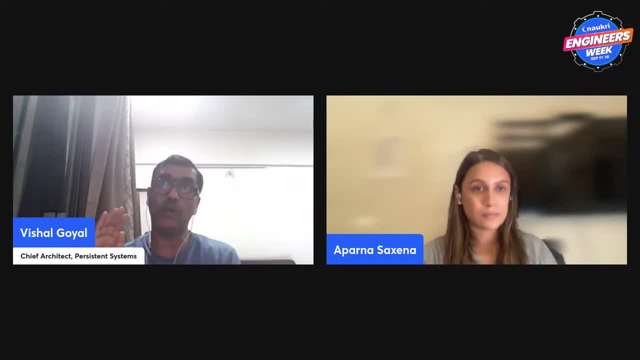 and things like that. But for people who come with hardcore, strong development background or who want to build a career in development and not necessarily get into data science and machine learning, start doing prompt engineering, start doing all those courses which I mentioned, start understanding.